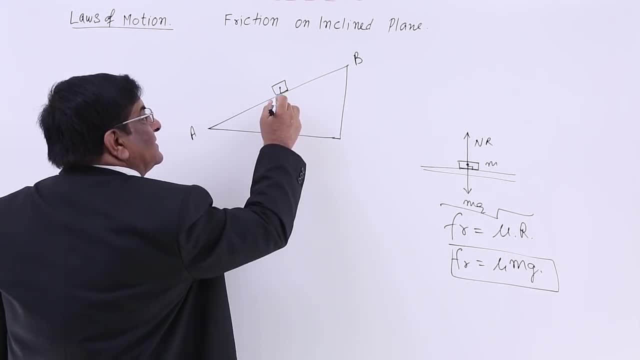 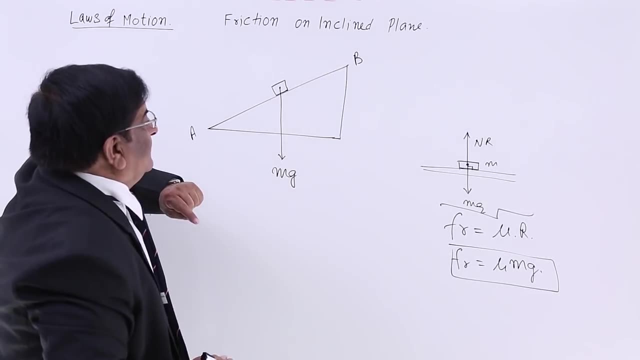 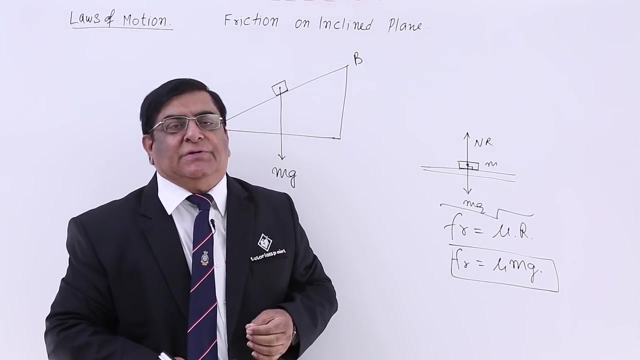 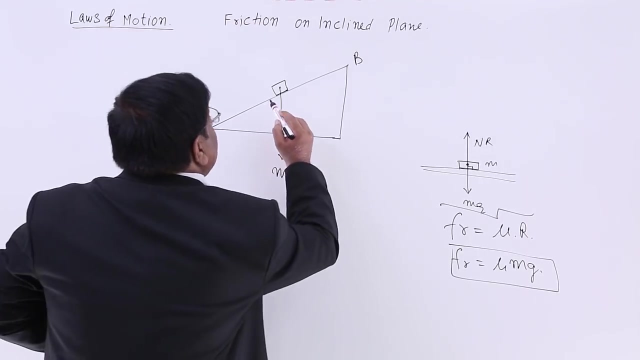 Now, when this applies the force here and there is an obstruction in the form of this surface, it is pressing the surface, The surface is applying a force on it. Now, any surface, when it applies force, it can apply force normal to it, normal to itself. Now, this is the direction. 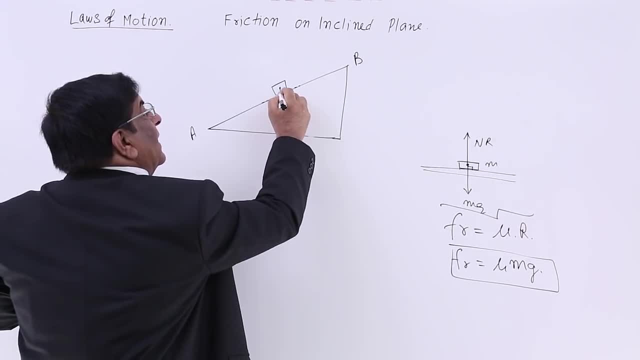 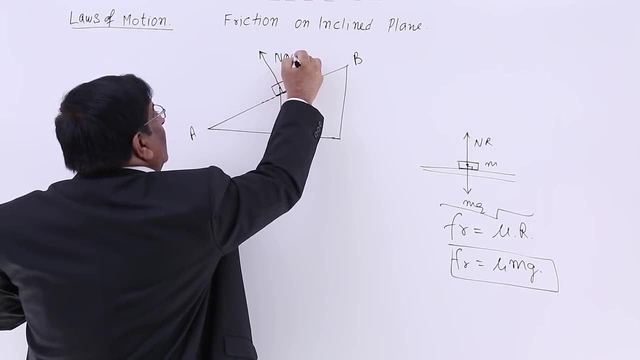 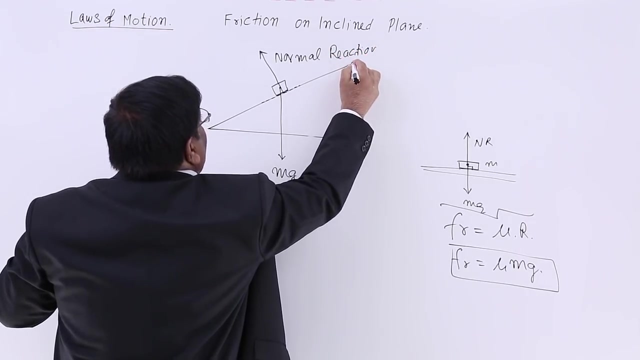 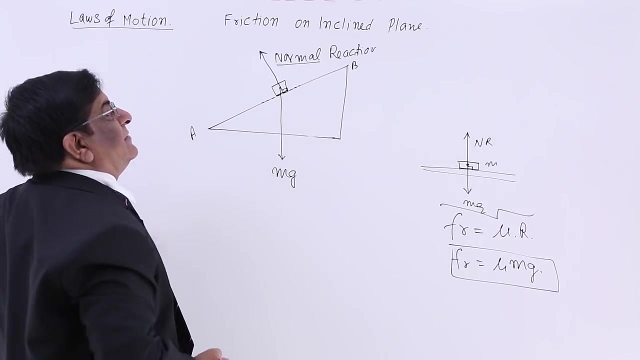 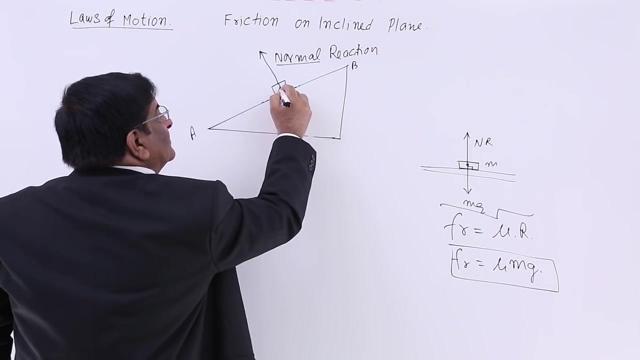 of the surface and it applies force in this direction. So this is normal reaction. Now, this is normal reaction. This is normal reaction here And because normal, so we have to make a 90 degree and then make a reaction. So this is normal reaction by the surface. This is. 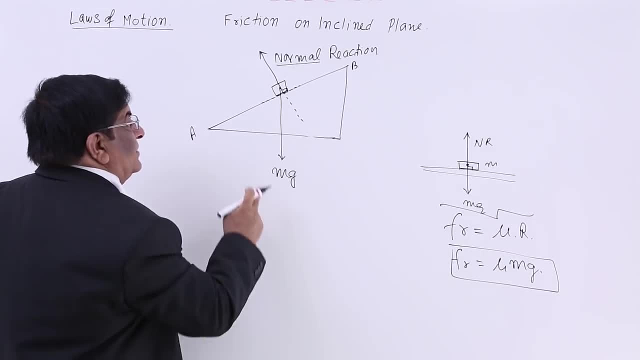 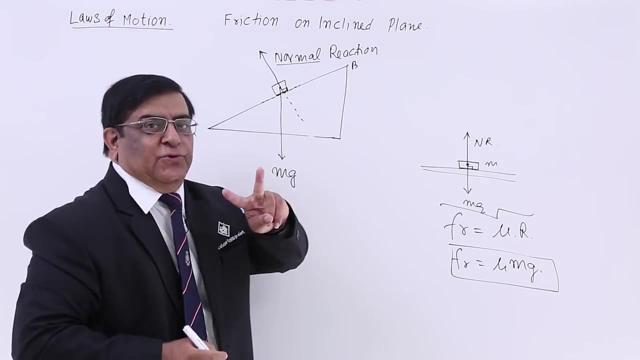 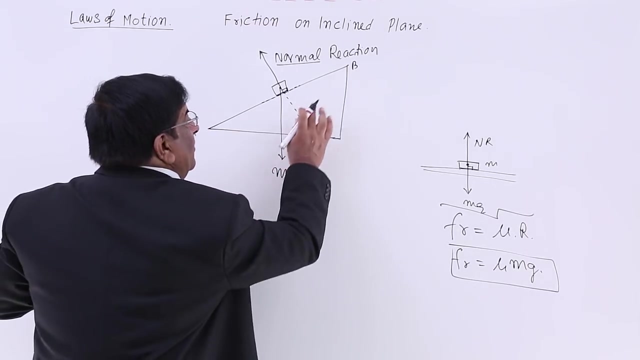 the direction of normal reaction. Now, this mg can. this is a force. This force can be divided into two forms. So there are two forces at right angle to each other, And we know that how we can divide a vector. So we resolve this vector into 2 directions. One is this direction along this: 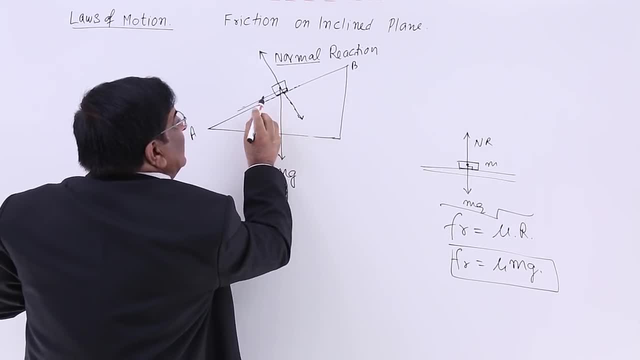 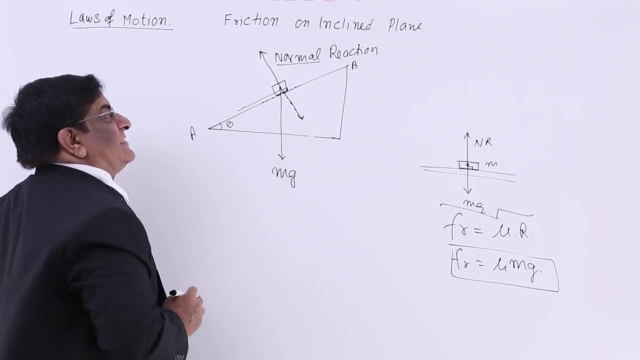 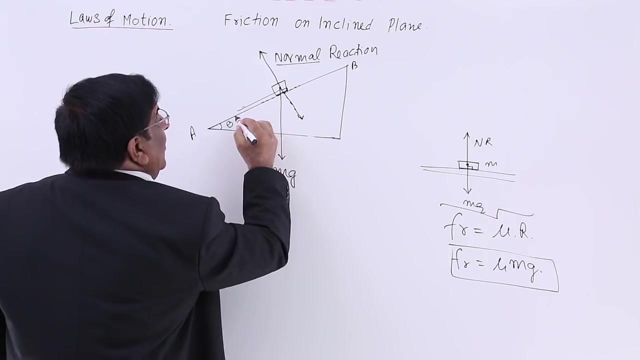 line, and one is this direction, which is at right angle to it. Now, we are trying to find out this angle. Let us take this angle, theta, This is the angle of inclination. Now, on this line, this is perpendicular. on this line, this is perpendicular. Therefore, angle between the two lines is equal to the. 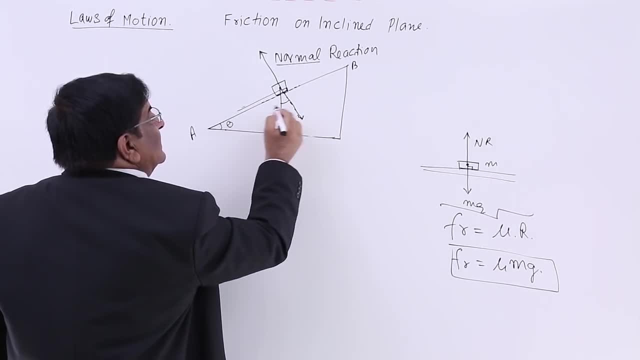 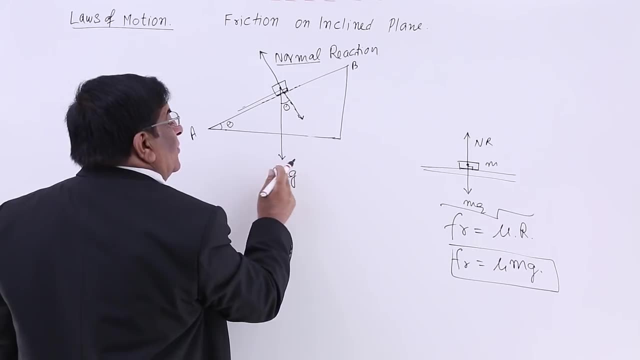 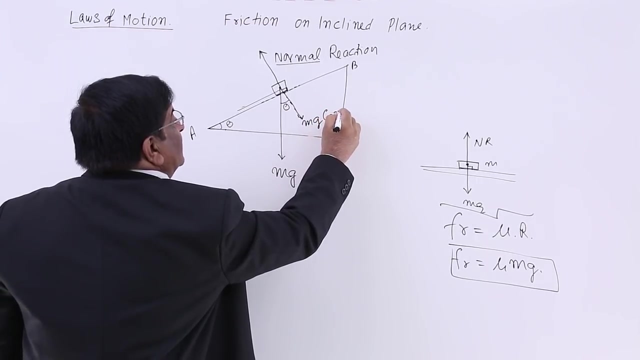 angle between the two perpendiculars and with this theory, this is also angle theta. Now, if this is angle theta and this is the force mg, the component of this force, mg, by the angle theta will be less than mg and this is equal to mg cos theta. This we have done. 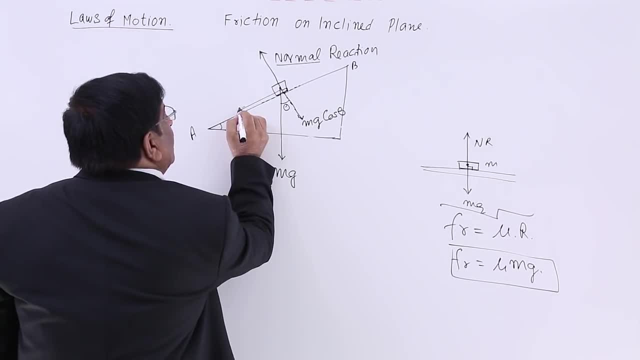 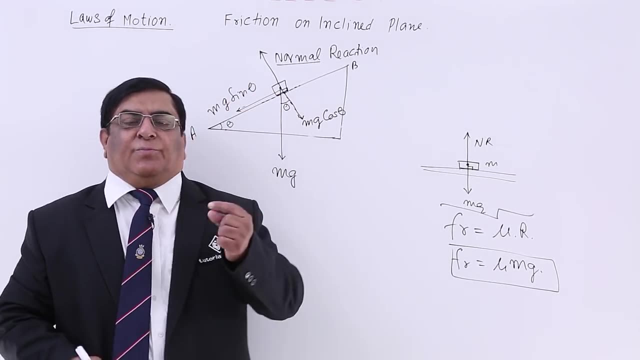 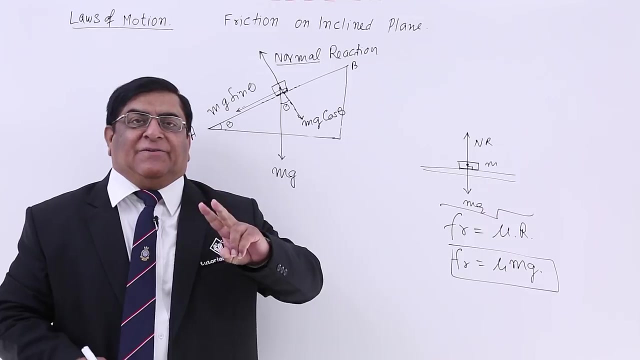 in vector resolutions. Now, the other component of this mg is mg sine theta. Now, what is meant by the components? Components, that mg which is acting due to gravity of the earth. we can consider as if there are two forces acting in place of one mg and they work in. 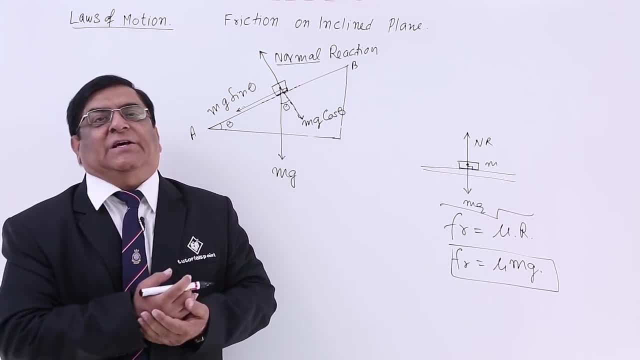 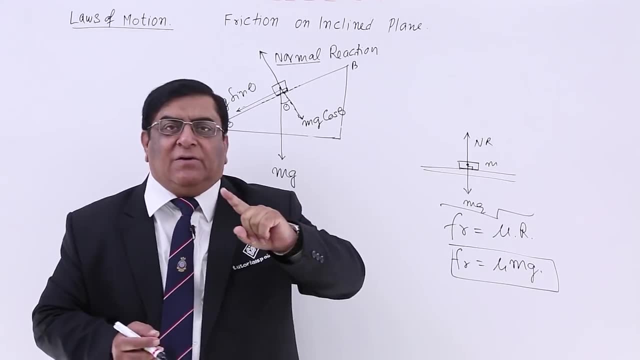 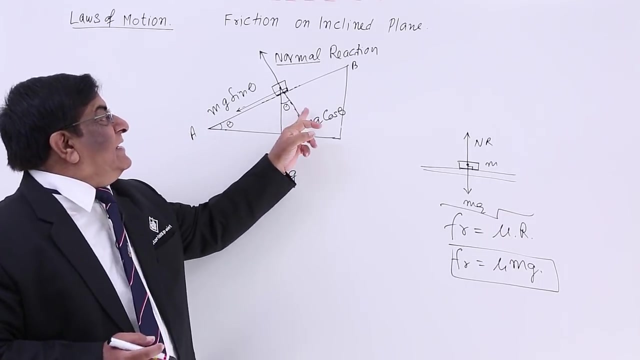 the directions where we need them to work, where we want their calculation, and we want their calculation in this direction as well as in this direction, because whenever we resolve, we have to make two components at right angle to each other, So that their sum is mg, because the total 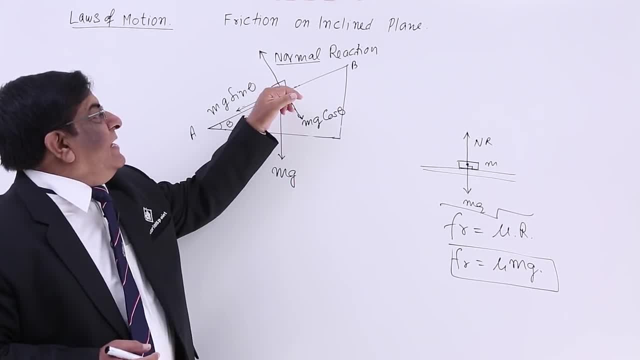 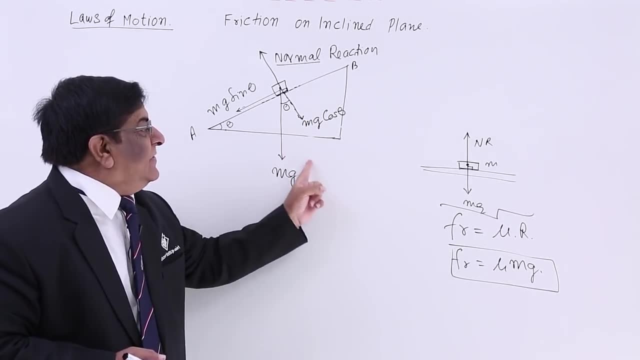 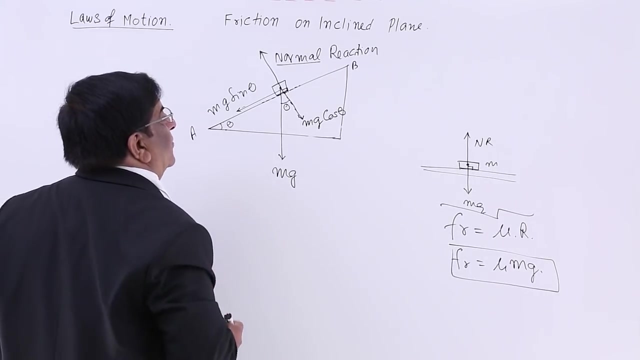 force is mg. it is not possible that we take only mg, sin theta and forget it. no, we have to take both. then only, we have taken cognizance of mg. ok, So mg is divided into two parts, because their sum is mg. Now these are the components. now what these components are doing. 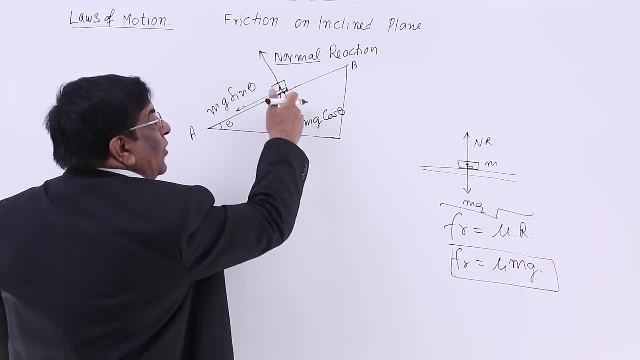 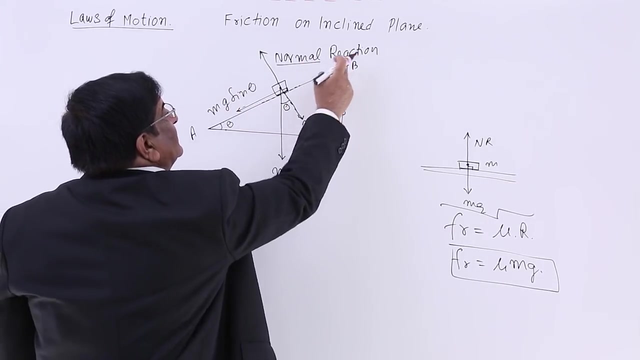 mg cos theta is pressing this surface at normal direction and in reply to that, this surface, according to third law, is pressing this object outward. So this mg cos theta generates a reaction which is normal reaction because it is at right angle. Now, on this body, mg. 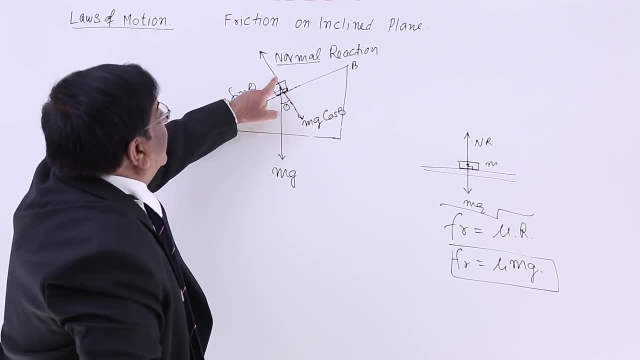 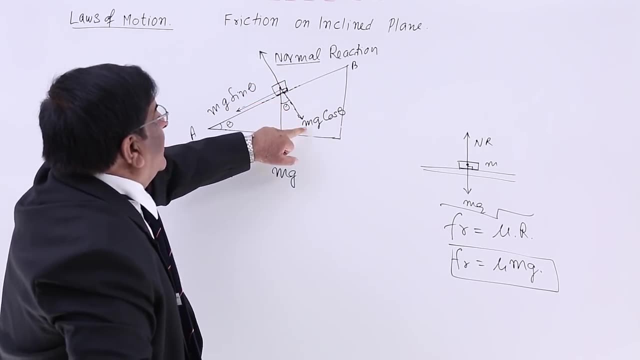 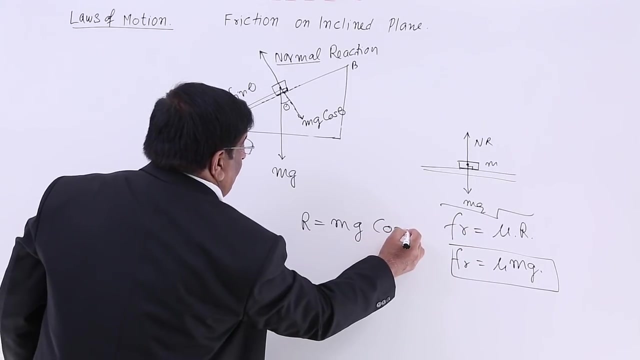 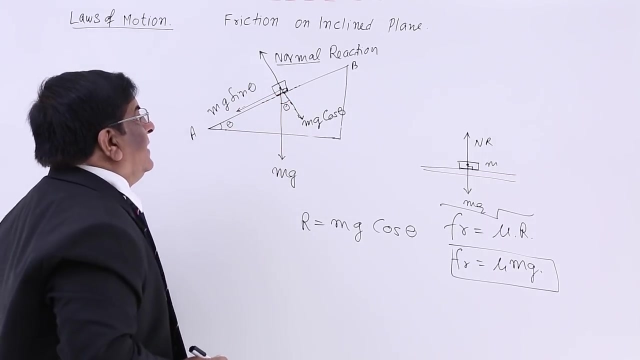 cos theta is So acting in this direction. normal reaction is acting at this direction and this body is neither going up nor it is coming down. that means this normal reaction R is equal to mg cos theta. ok, Now we come to this mg sin theta. mg sin theta is in this direction. 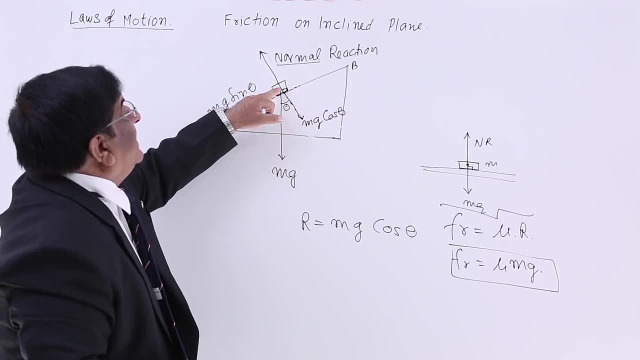 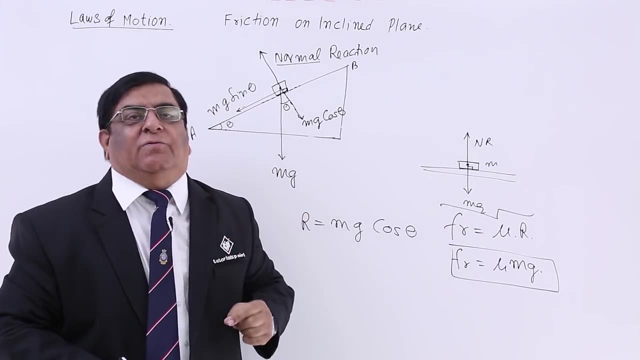 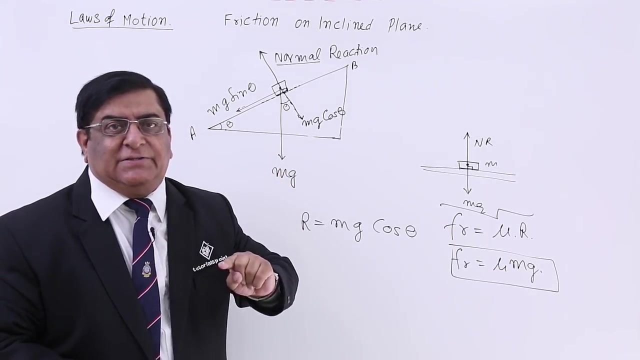 if there is no force to balance it, then this will slide down, This will move, It will become a unbalanced force. So one thing you should always remember: that which component of the mg, which component of the weight, is responsible for moving the object. 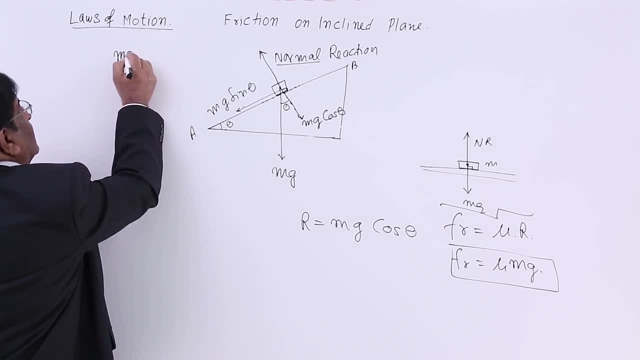 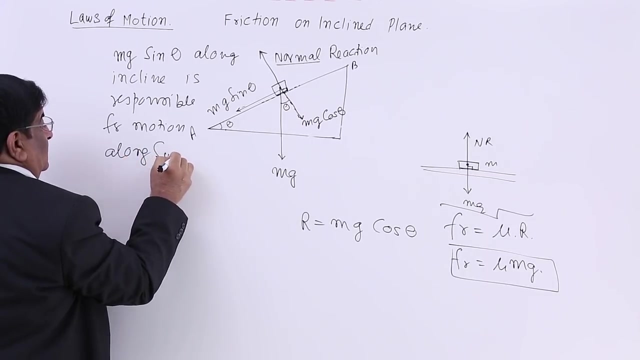 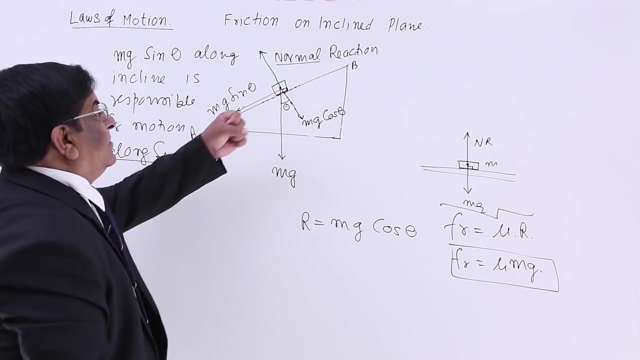 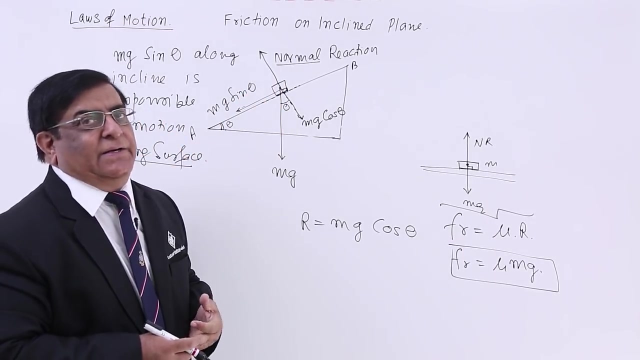 So I will write it here: mg sin theta along incline, responsible for motion along surface. So please always remember it: when this is angle theta, then it is m g sin theta which trying to bring it down. Now, if nothing balances it, then it will pull it down, but the moment a motion start, according to our principles, 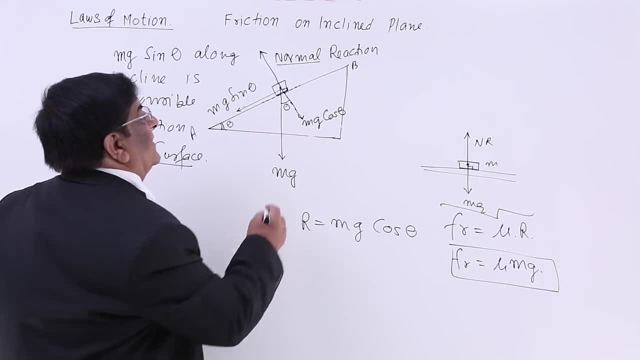 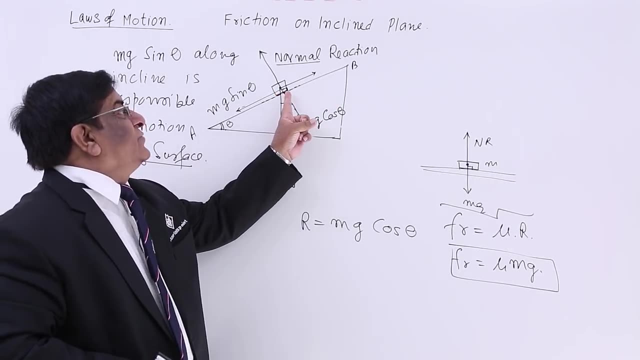 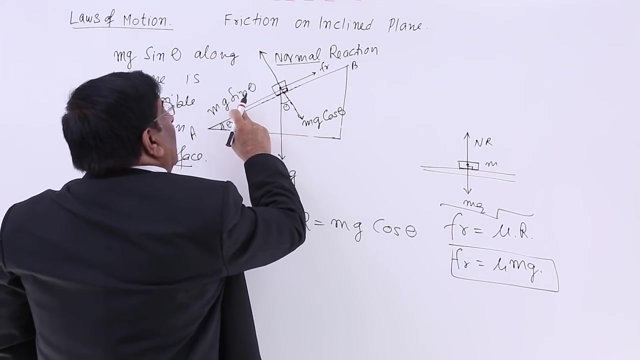 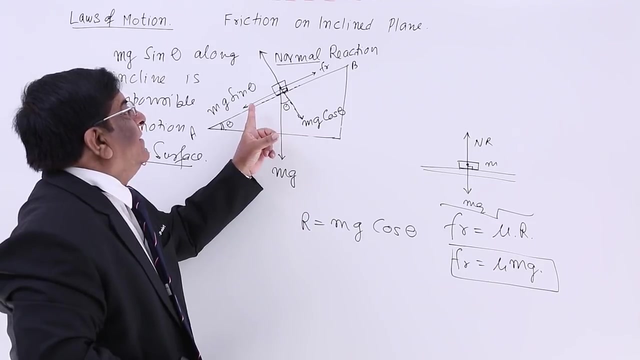 and knowledge. a friction is developed between the two and that friction is trying to stop it. Now, if the friction has succeeded to stop it, then what does that mean? That means the friction is equal to m g sin theta. If friction is equal to m g sin theta, then it: 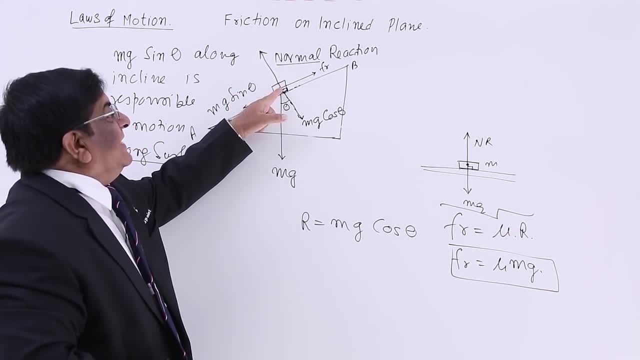 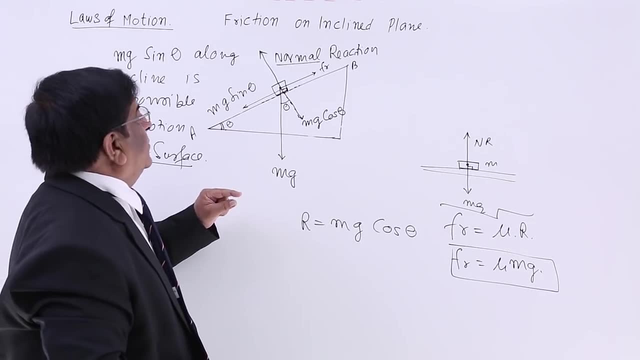 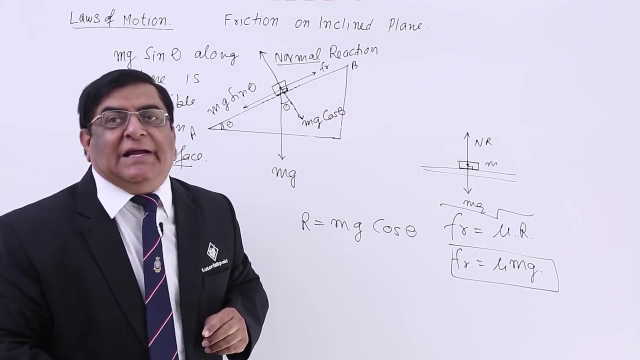 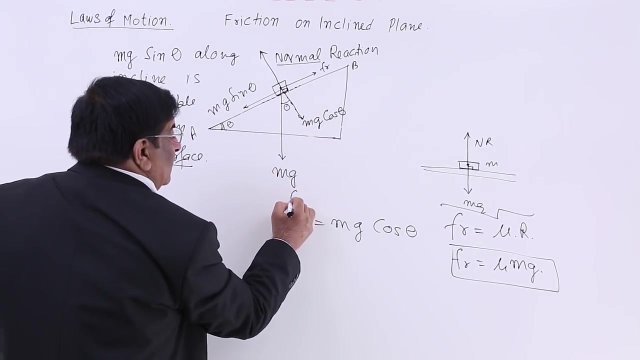 will stop and it will stay. no motion will stop The submission there also same the parecer, which you can read it, and it has no movement anywhere. We think that pain situation can only heave, recover and thought the situation can be move with the porsche ready setting and the next set of senses, and also it is. 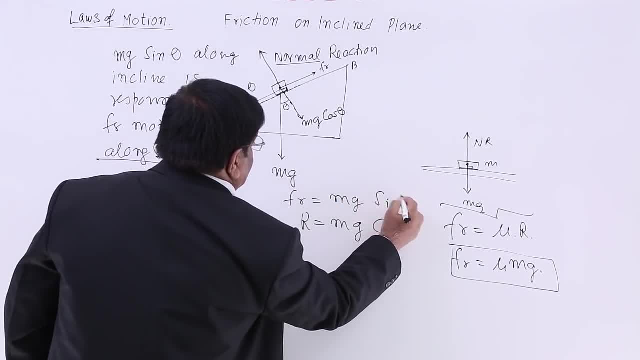 thin, and so in order to make the porsche able form porsche body, it has to be made pretty small. in speed they are of scale. Any jaws probably win or there will beンフ salvation for porsche. The force is balanced. Now suppose this is the condition when it is at the verge of starting. 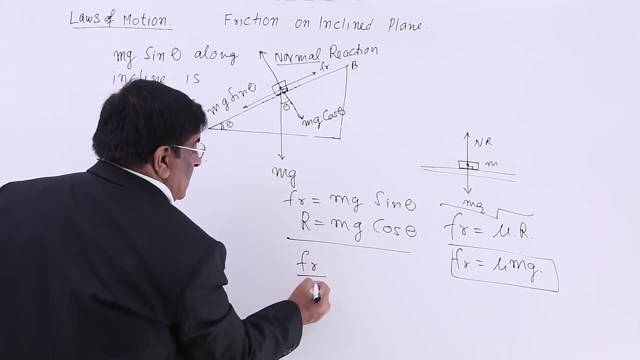 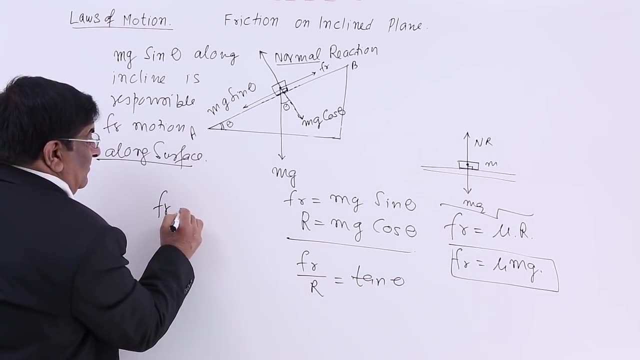 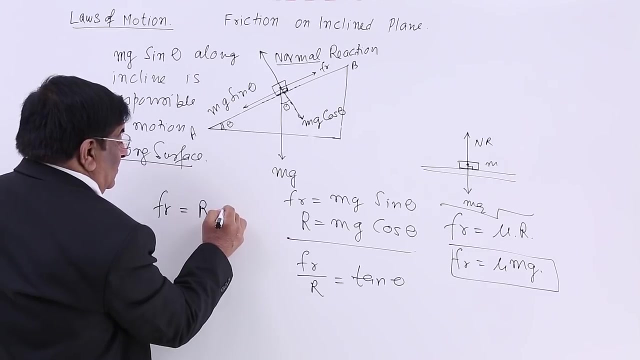 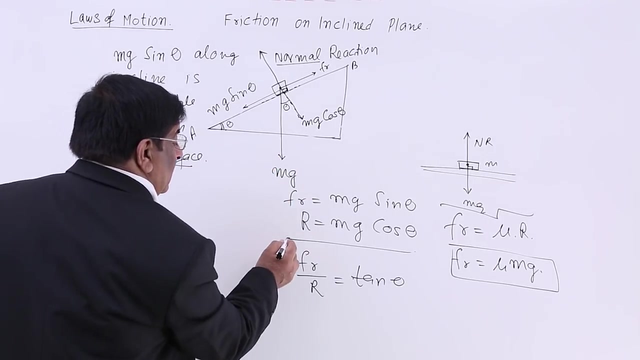 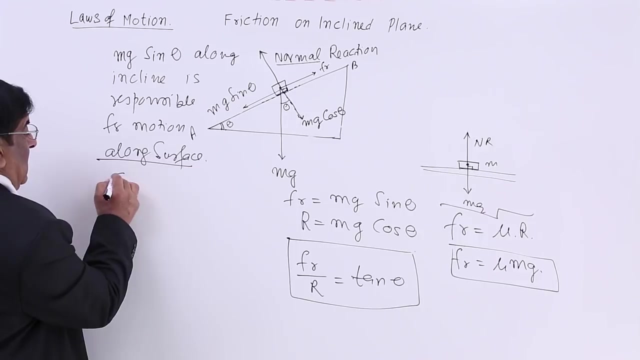 we have friction. normal reaction is equal to tangent theta. so friction is equal to normal reaction. sorry, yes, normal reaction into tangent theta. no, we are not going to do that. we want to find out tangent theta and this is tangent theta. now, here, when the body will slide, what? 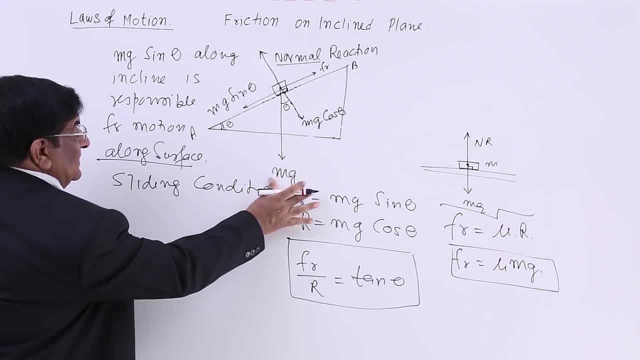 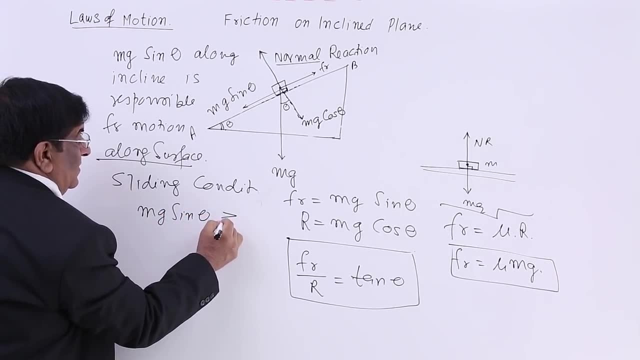 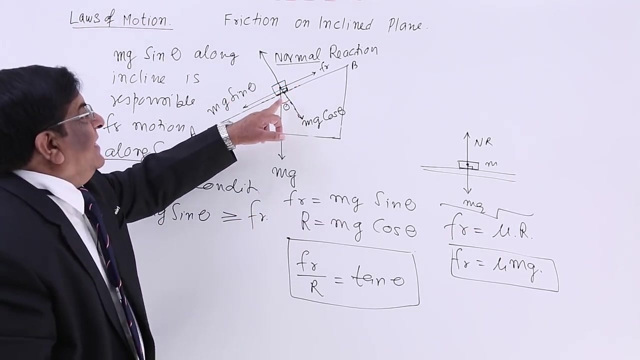 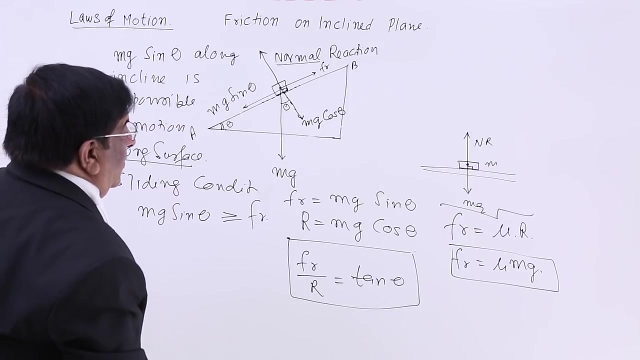 is the sliding condition. the sliding condition is when mg sine theta more than friction. ok, So this is the sliding condition. If this become larger than friction, then this will slide down. ok, right Now. what is the net force with which it will slide down? 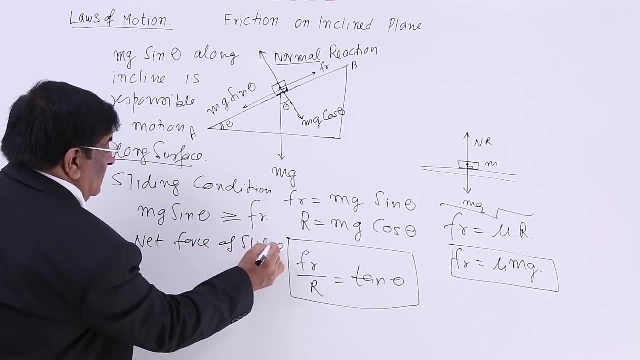 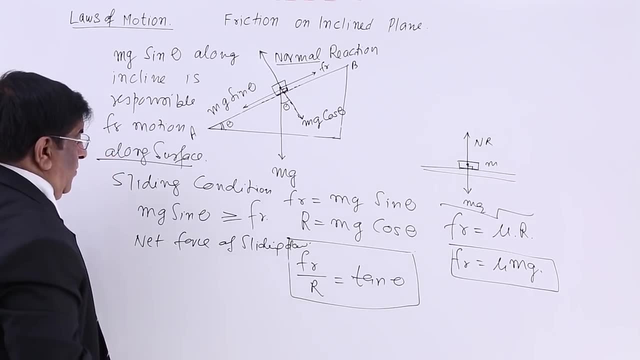 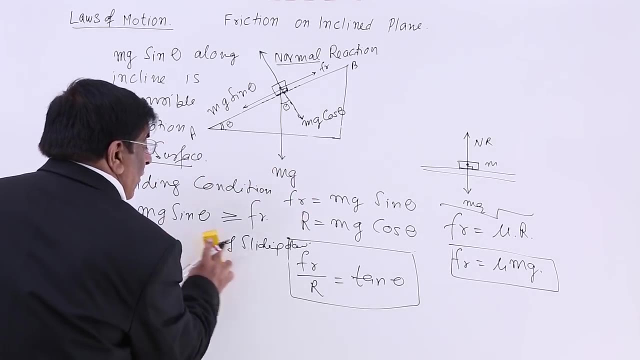 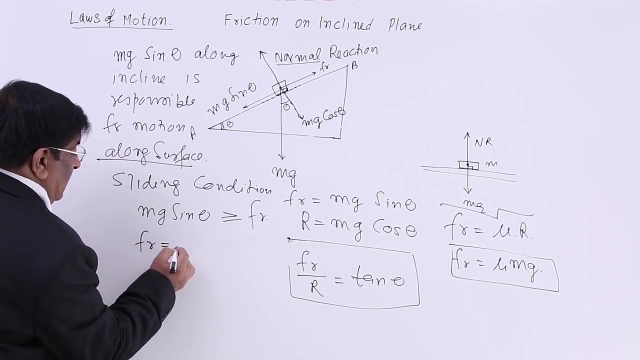 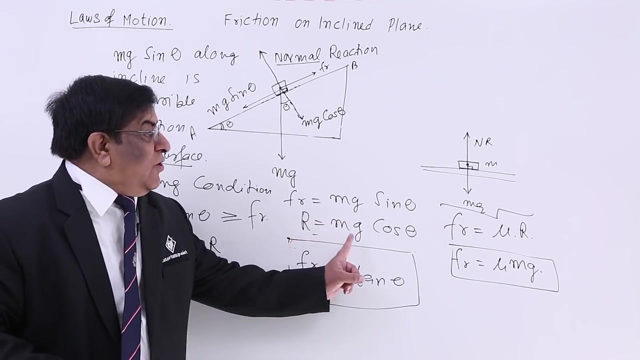 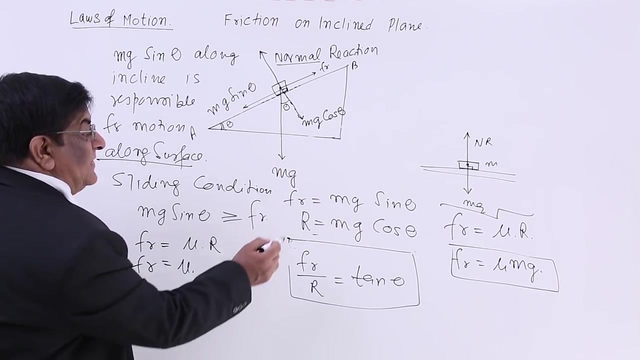 Net force of sliding down. Ok, first, we know the friction as a relation with normal reaction. friction is equal to mu into normal reaction. in this case, normal reaction is this: in this case, normal reaction is not mg. In this case, normal reaction is mg, cos, theta, this we have done it ok. so if this is normal, 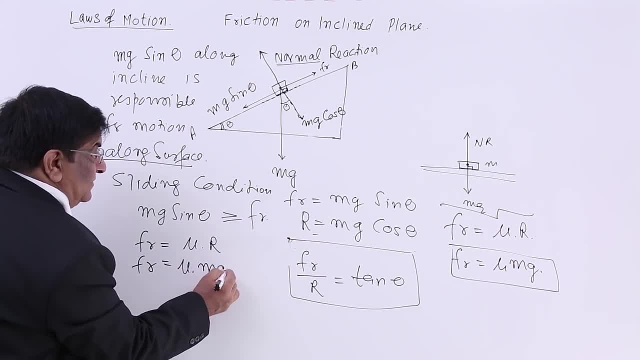 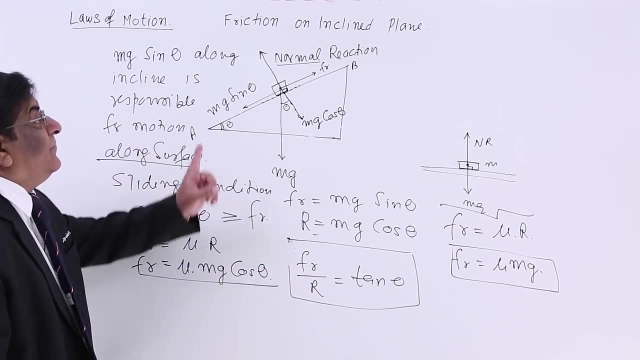 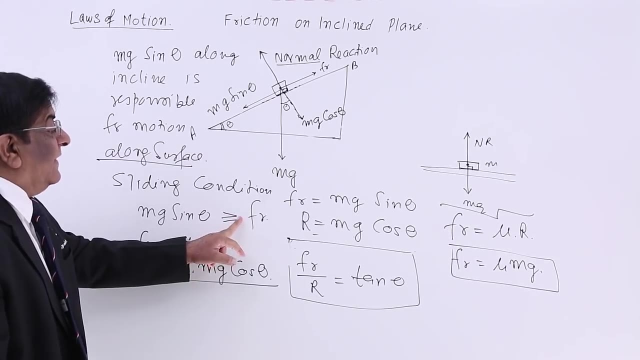 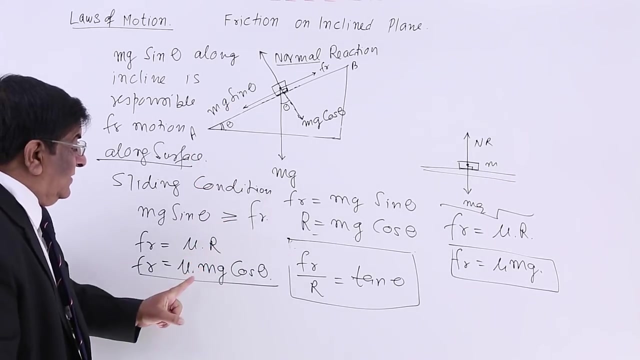 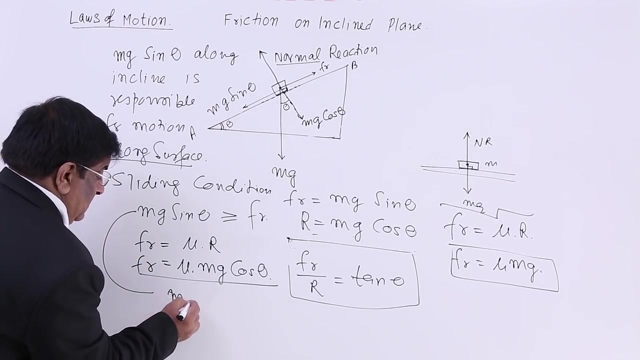 reaction, then I will write it here: mu: mg cos theta. this is the friction. Now what is the condition for sliding? mg sine theta should be more than the friction. that means So mg sine theta should be larger, equal or larger than mu into mg cos theta. mg sine theta. 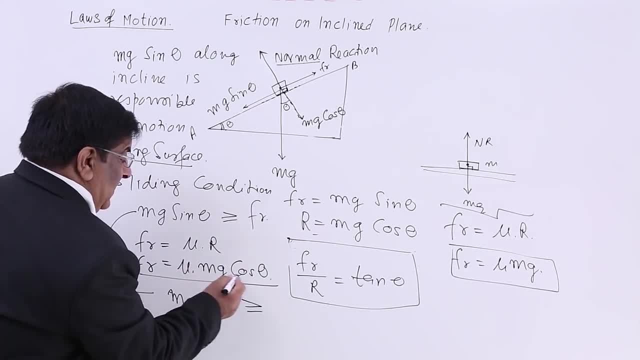 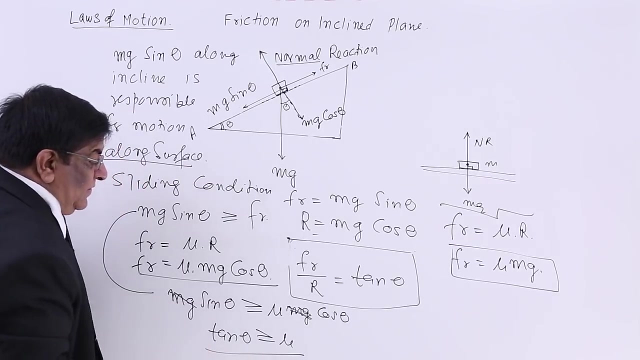 should be equal or larger to friction and write value of friction here mu, mg cos theta. here mg mg is cancelled, So sine theta should be larger than mu cos theta. Ok, Take cos theta here, this will be tangent theta. yes, so if tangent theta theta is so large. 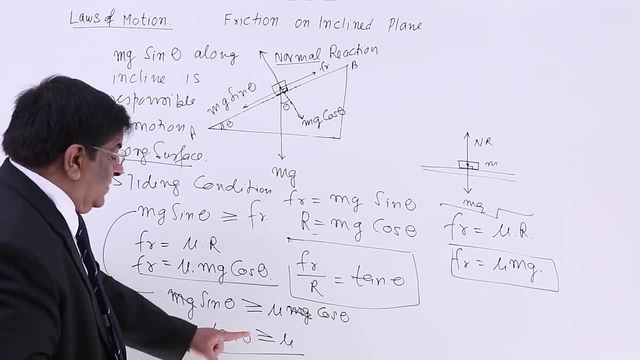 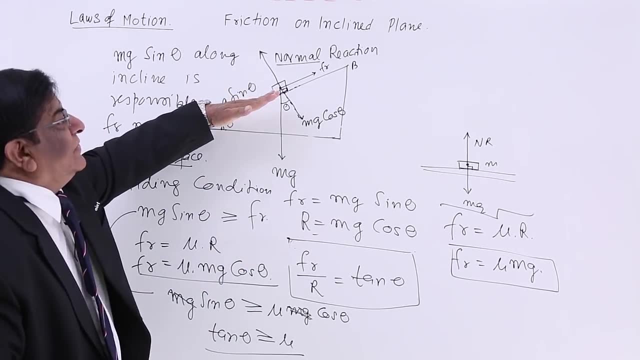 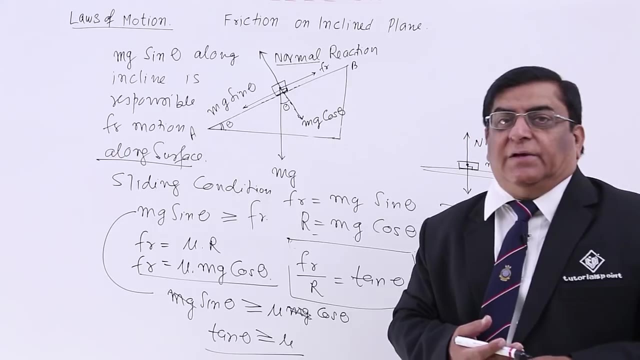 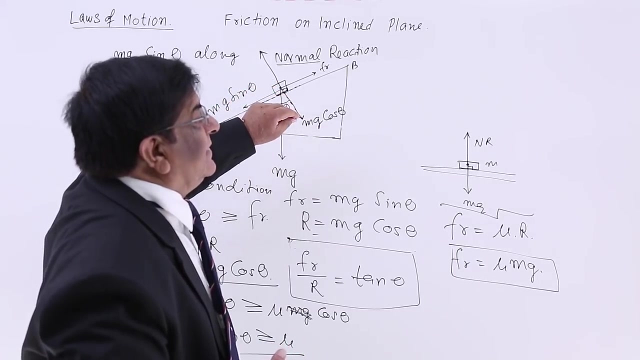 that tan theta is equal or larger than mu, then the body will start sliding down. this is the friction on the inclined plane, and this we have already done when we were doing angle of repose. ok, Ok, Now how much? if there is a such situation, then how much force is required to push the? 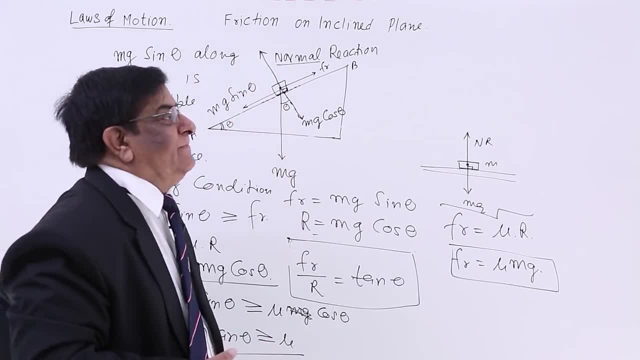 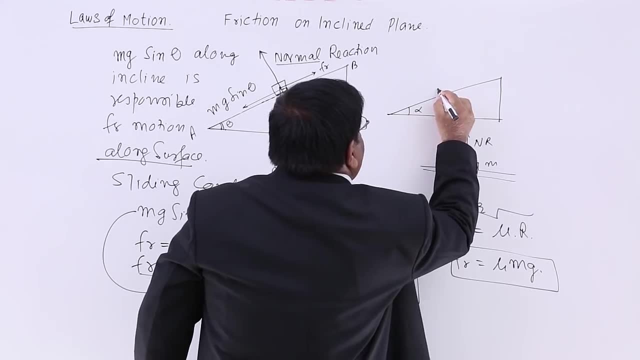 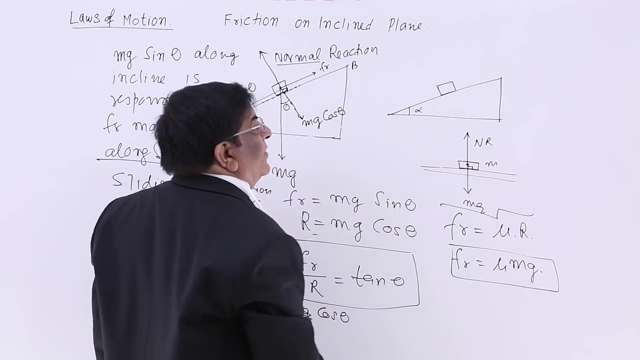 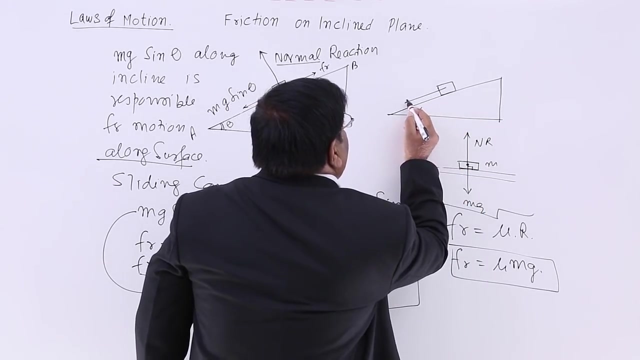 body downward if it is not sliding. ok, I push a body here, I keep a body here and I see it is not sliding down. Why? Because I know there is a friction here. that is why it is not sliding down. So I apply a force here. mg sine theta is acting on it. here is friction. how much is? 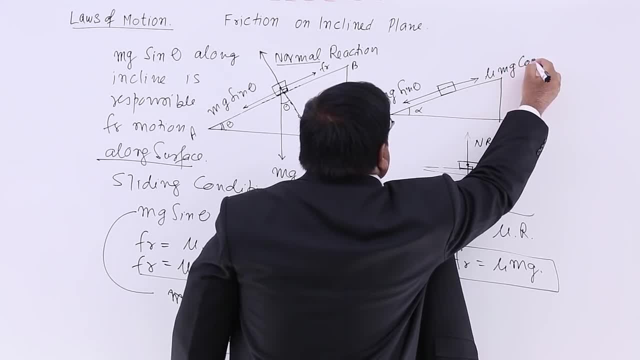 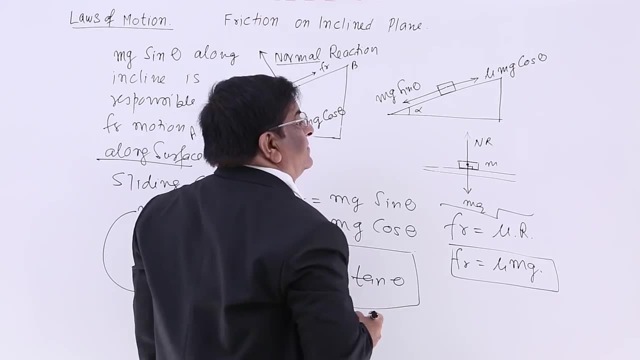 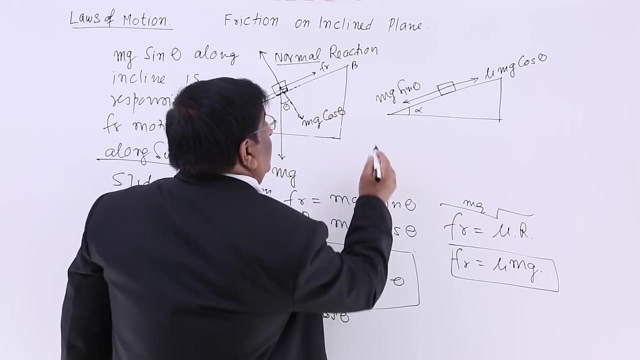 the friction friction is mu mg cos theta. this we have already done- friction. Now, if it is not sliding down, then I have to apply an additional force on it. Ok, So that it will slide and I apply a force here. that force is F. now it starts sliding. 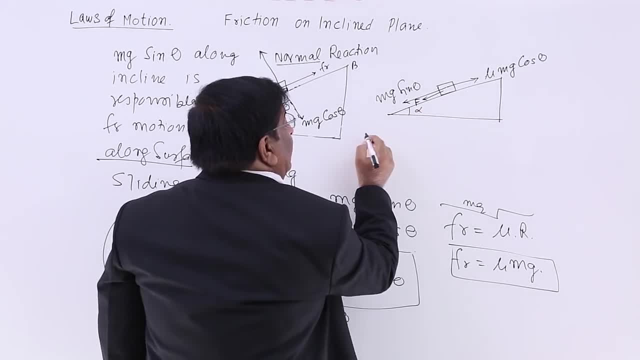 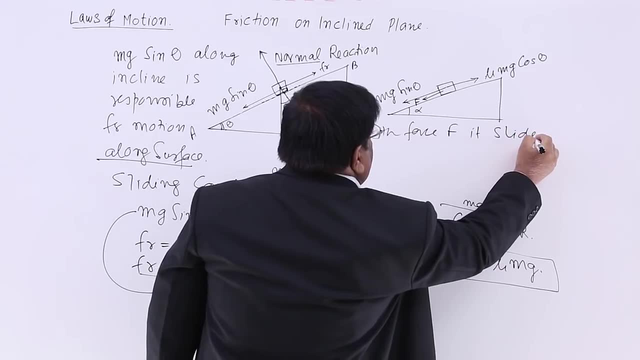 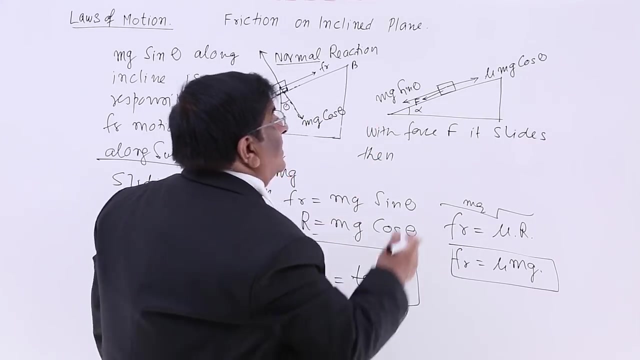 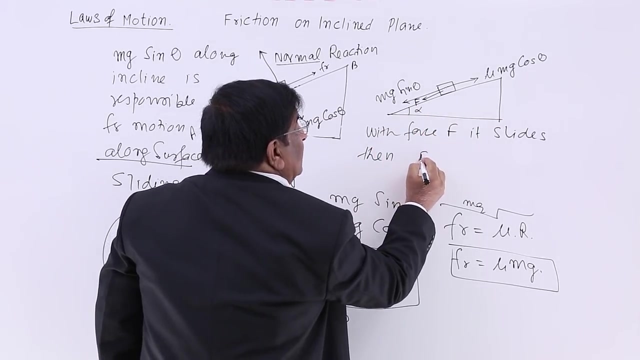 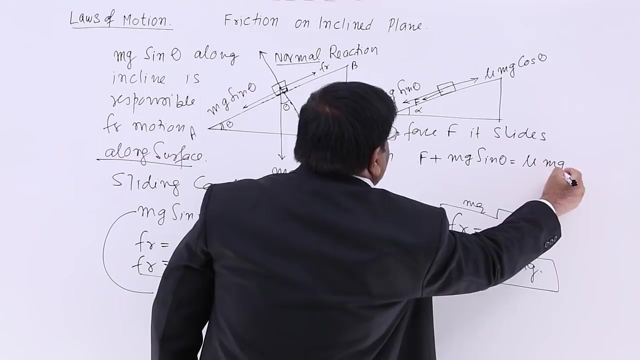 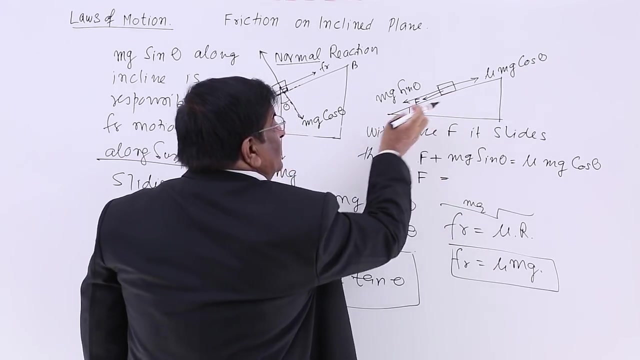 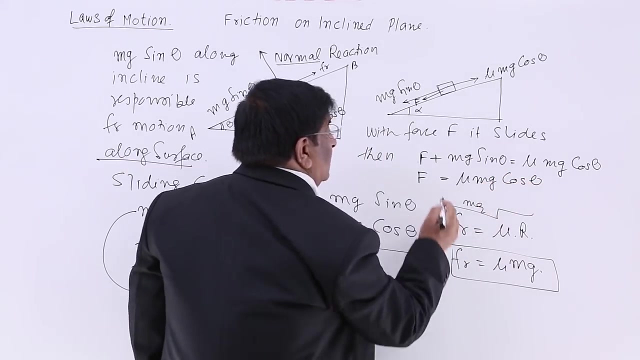 I want to find out how much is this force which is required to push? pull it down, then F is equal to Ok. since it has started sliding down, I can write that F plus mg sin theta is equal to mu mg cos theta. So how much is F? The force required to pull it down is mu mg cos theta minus mg. 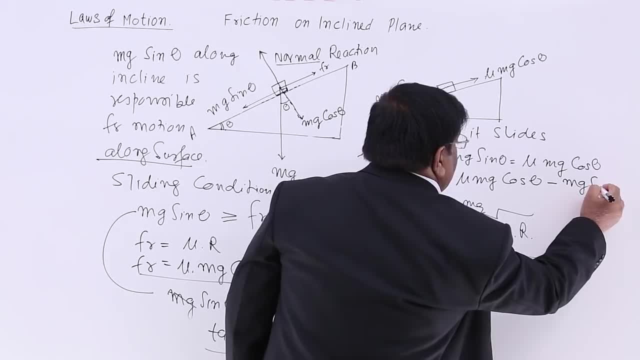 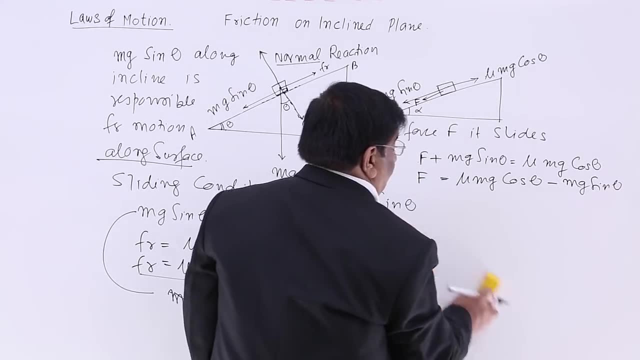 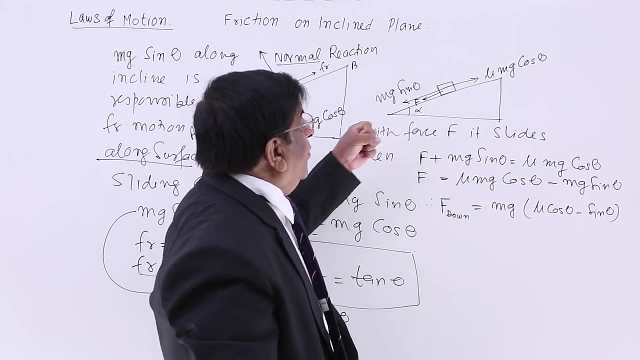 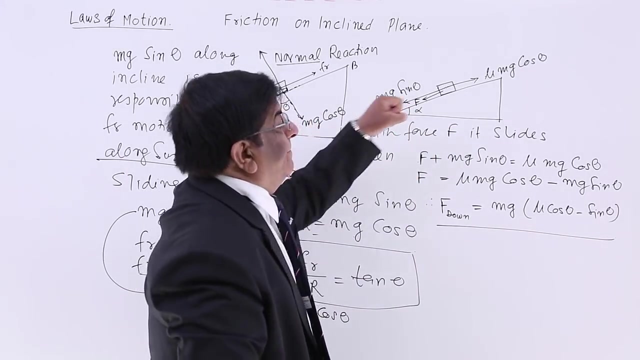 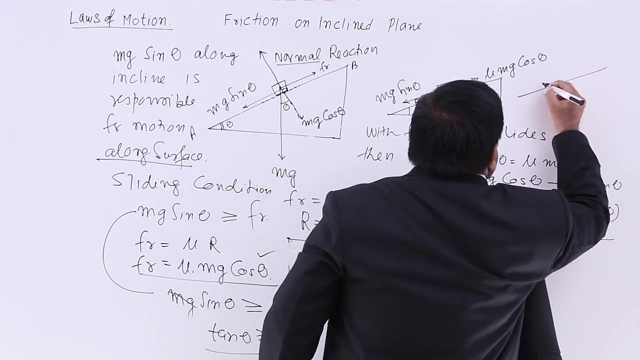 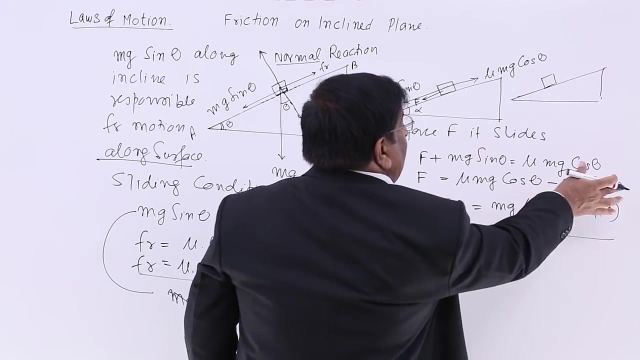 sin theta, You can take mg out. This is the force required to pull down. Now, second case: I want to push it up. If I want to push it up, then the situation is here. This is the box. Oh, this is angle alpha. Everywhere I should put alpha, No problem. 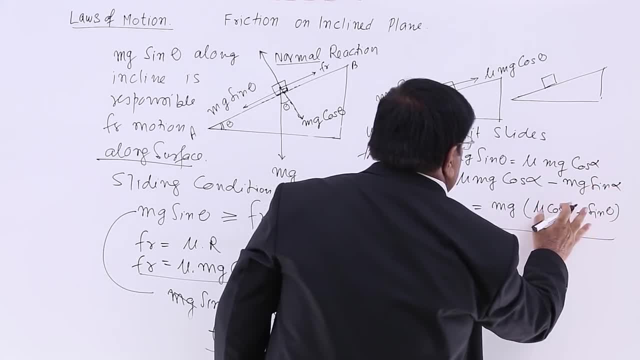 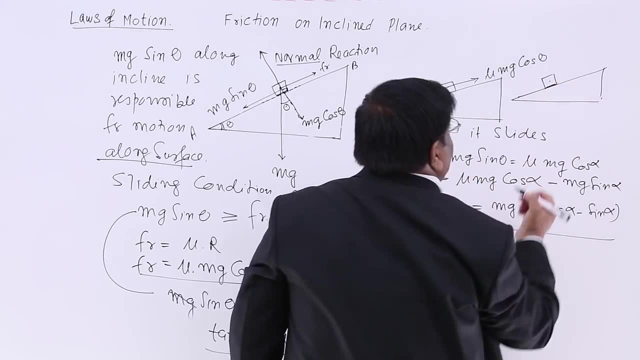 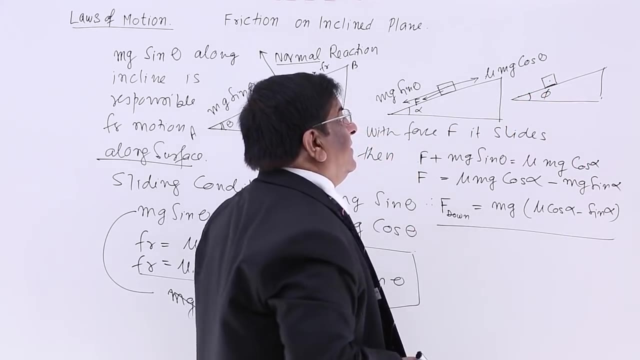 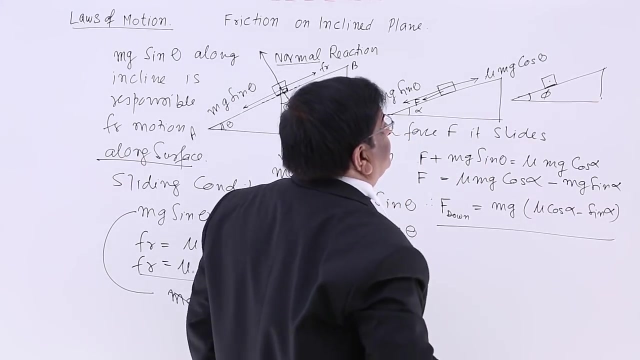 You can do that Now. here is an object. There is an incline with angle phi and I put a box here. It is at rest and I want to push it up so that motion starts. This is very important, please see. 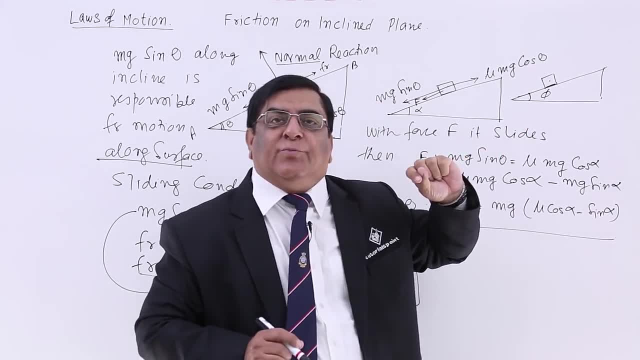 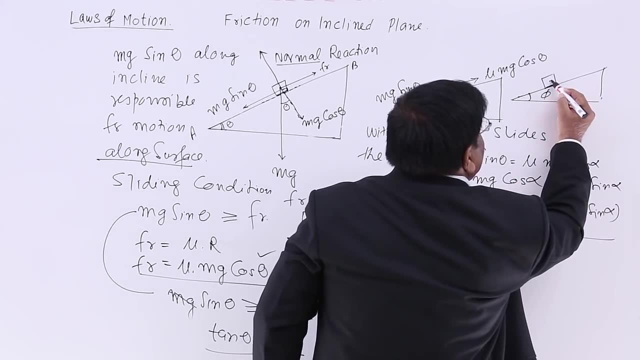 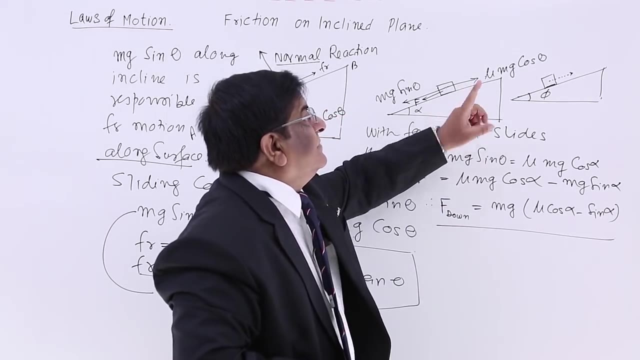 When I want to push it up. where is the intention of motion? Intention of motion is for upward motion. If I want to move it in this direction, then what will be the direction of friction? Will it be same? Answer: no. 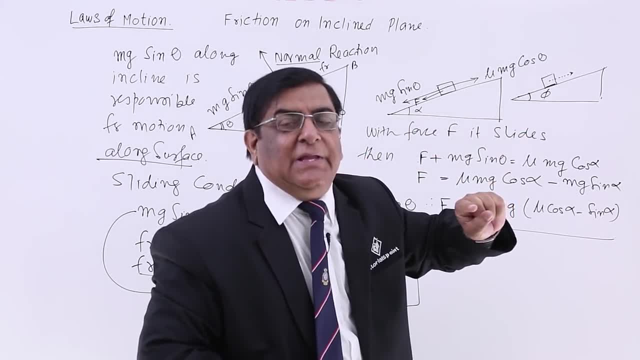 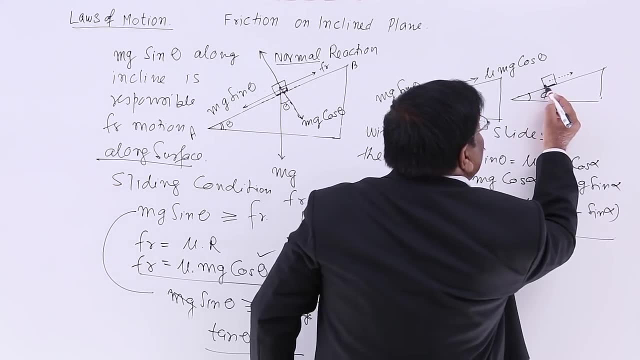 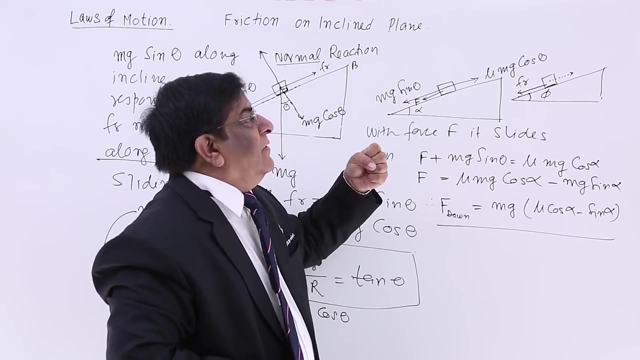 Because if I have an intention to move up, then friction will be generated in opposite direction of the intention. So in this case, here is the friction. See, in this case I am pulling it down. where is the intention of motion downward? 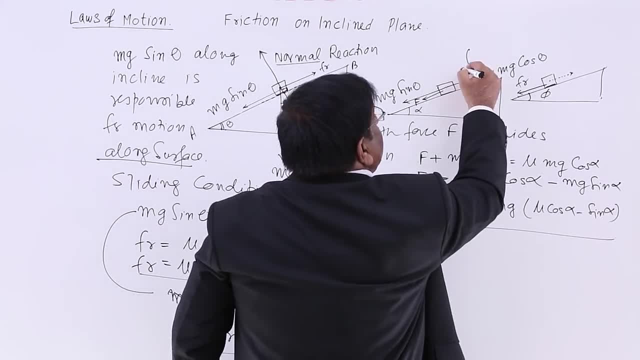 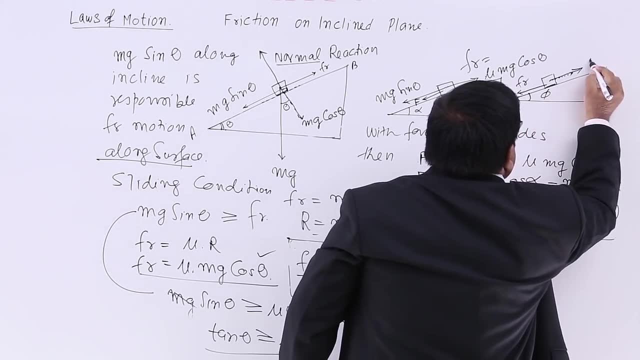 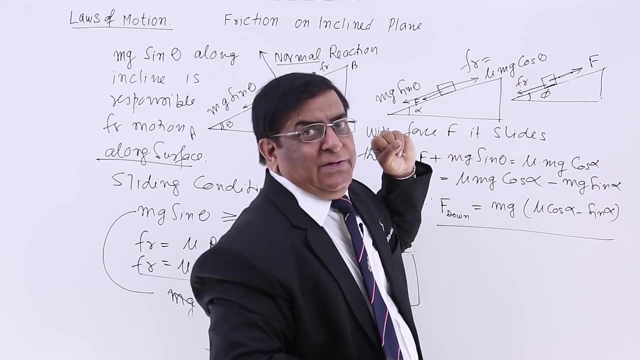 So where will be the force of friction? upward In this case. what is my intention? I want to push it up, To pull it up and I apply a force. where is the intention? upward. So friction will automatically be downward. 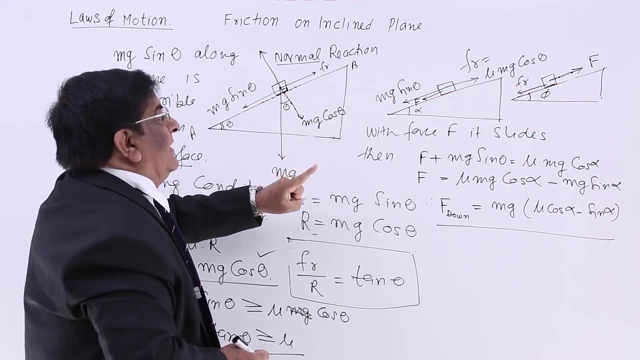 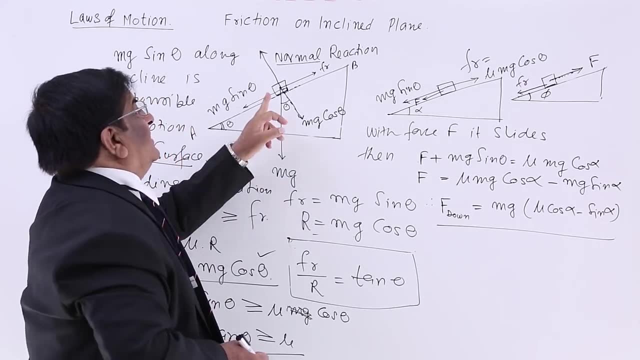 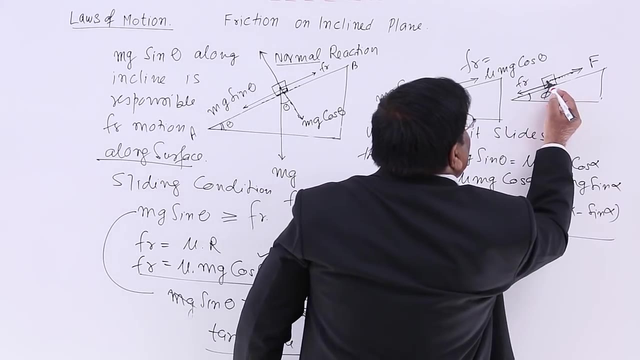 Now, because it is an incline. at every incline, Mg participate with a force, Mg sin theta, in this direction, Whether it is going up, whether it is going down, the component of Mg in this direction is always Mg sin theta, and that is here Mg sin theta. 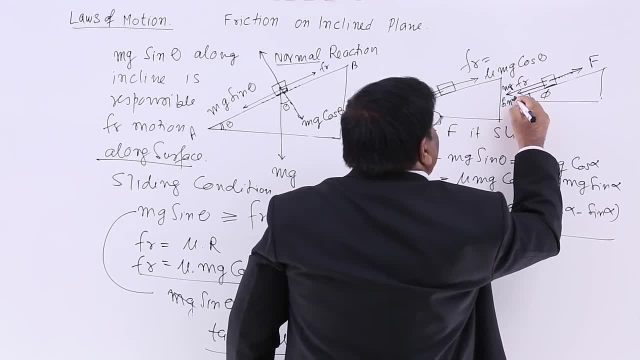 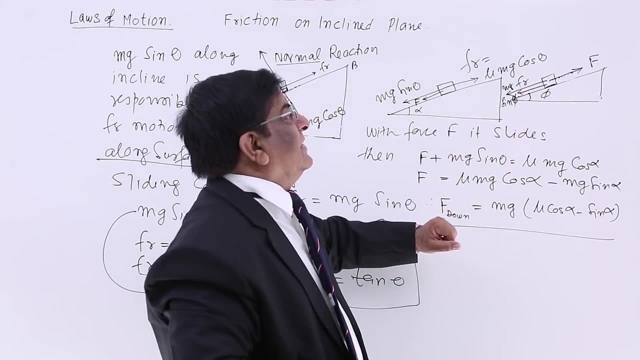 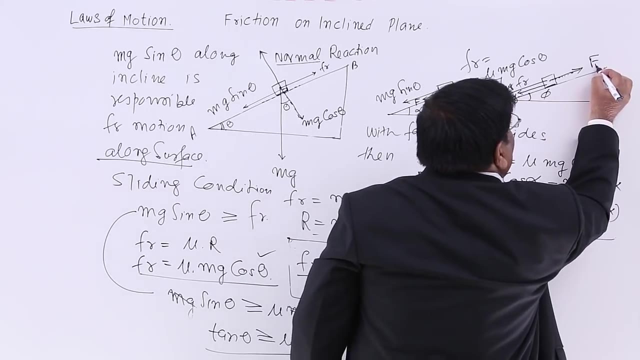 Okay, Mg sin, this is phi. so, Mg sin, phi, It acts in this direction. Friction acts in this direction. I am applying force in this direction because I want to push it up. So this is force for upward motion. This was downward motion. 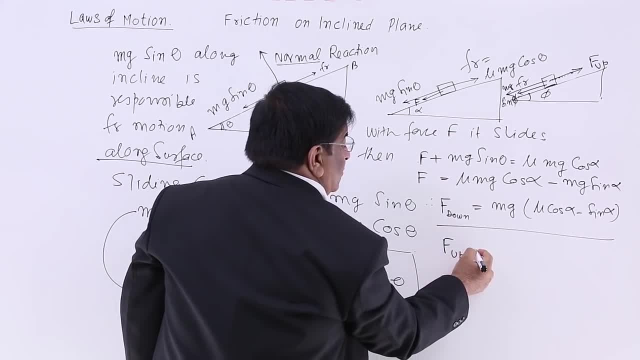 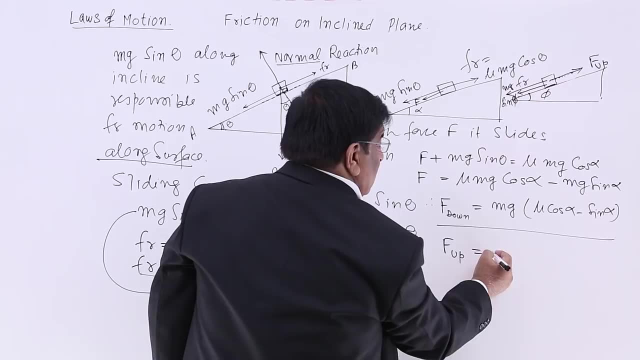 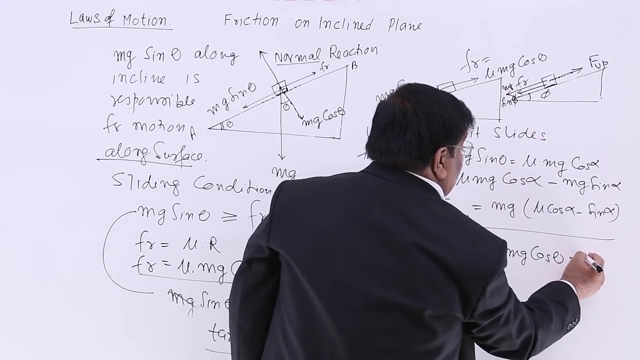 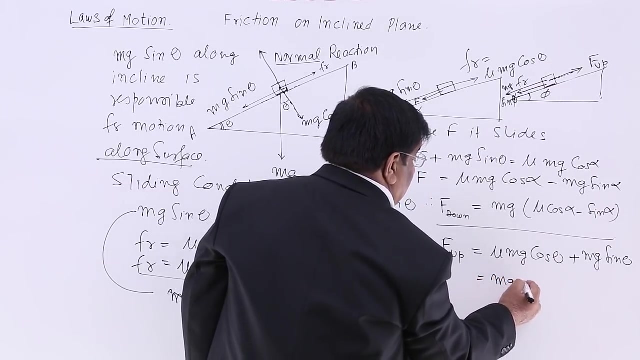 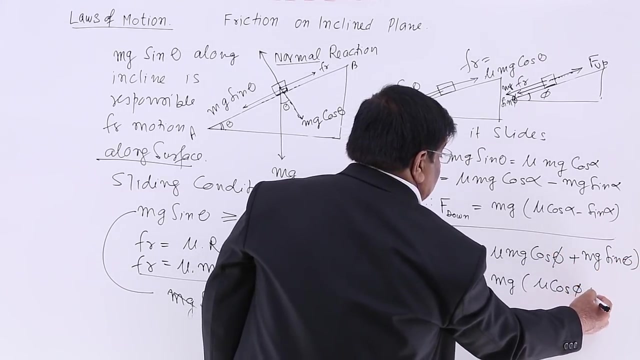 Now, what is the equation here? Force for upward motion, the incline is equal to sum of the two, That is, Mg sin theta, Mg sin theta, Mg sin theta. This is friction: Mu Mg cos theta plus Mg sin theta. And this is equal to Mg Mu cos phi plus sin phi. 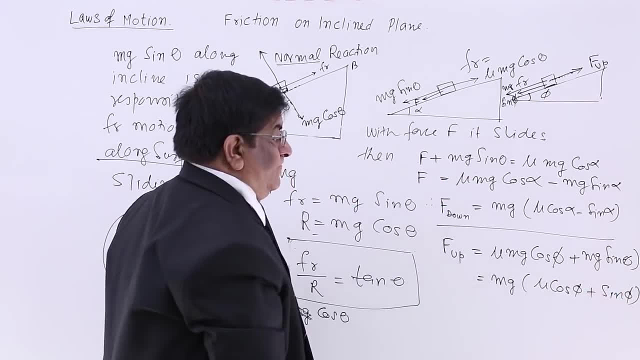 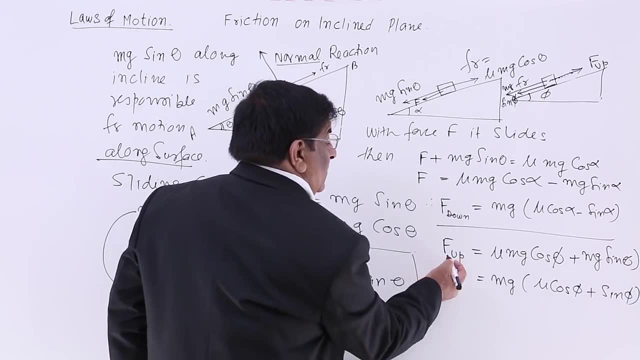 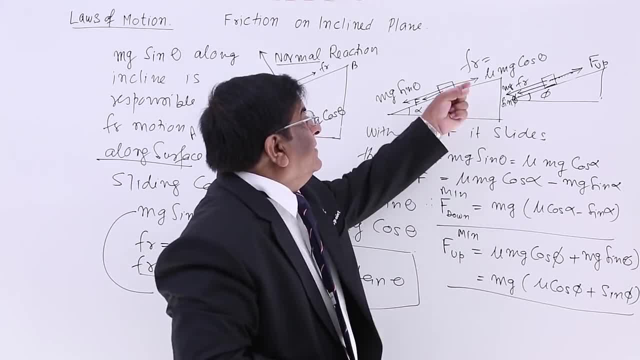 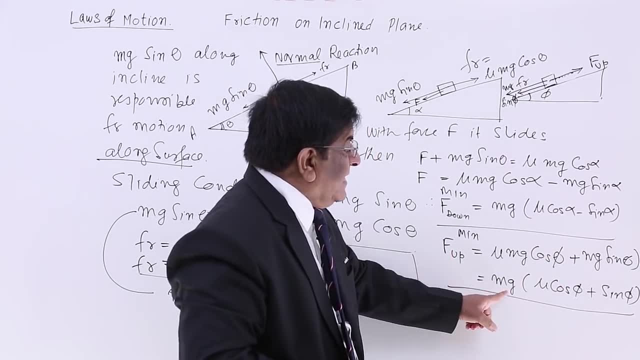 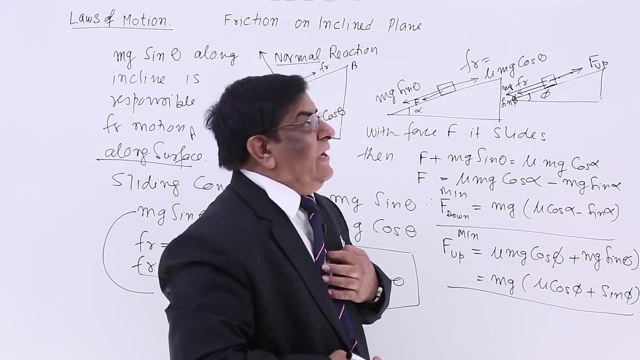 So minimum. See the minimum force required to bring down the object is Mg, Mu cos alpha, minus For taking up same Mu cos is there, but in place of minus this is plus Okay. Now say the value of Mu cos alpha: Mg, Mu cos alpha. 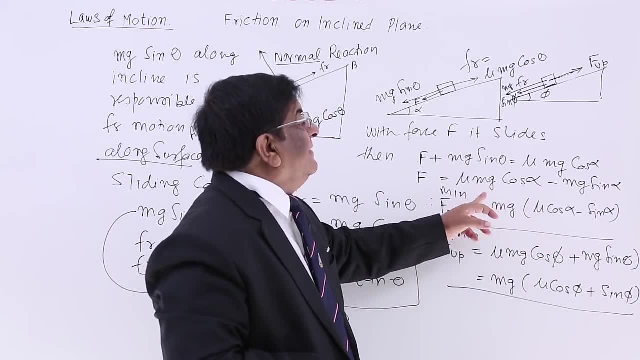 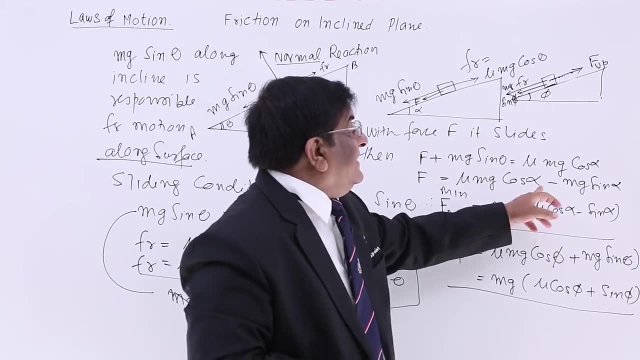 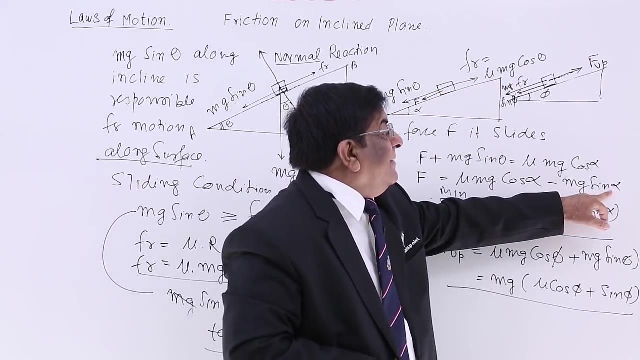 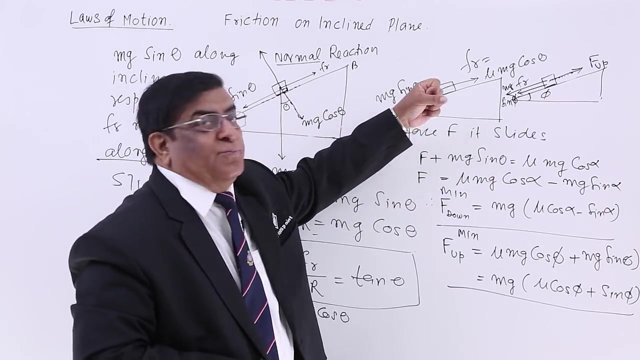 Minimum force required. Minimum force required, Minimum force required in a particular case is 100, and this is say this is 60. again, mu mg cos alpha friction is 100 and mg sin alpha is 60, 160. how much force I need to pull it down? yes, you know. 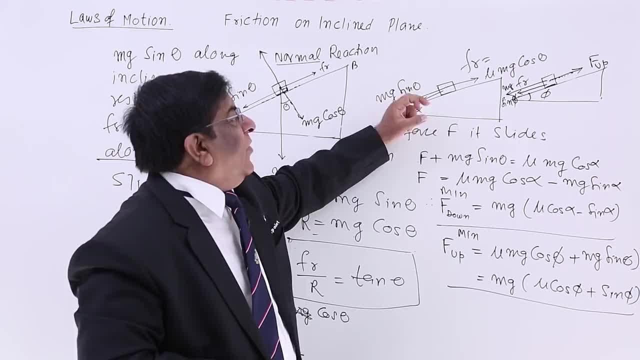 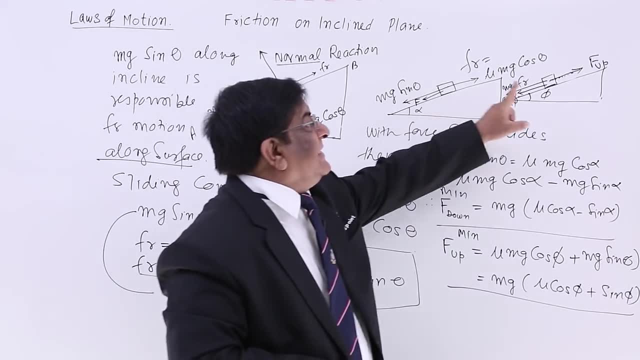 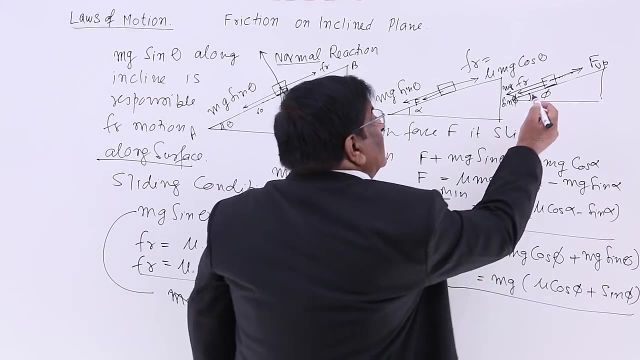 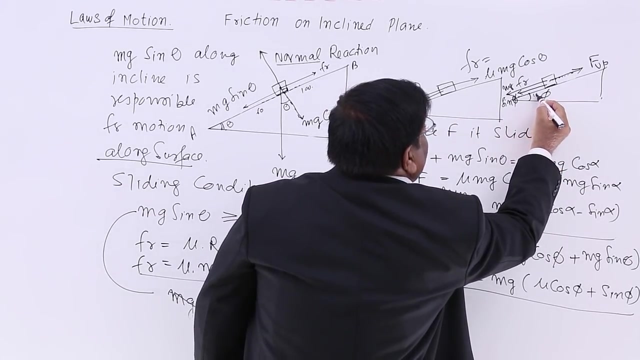 it will be 40, because 60 is friction. 40 I apply 100, 100 is friction and it will start sliding down. in this case, 60, 100. okay, in this case, the moment I apply force here, this 100 friction comes into this direction: 100. this is 60. so how much force I have to pull? 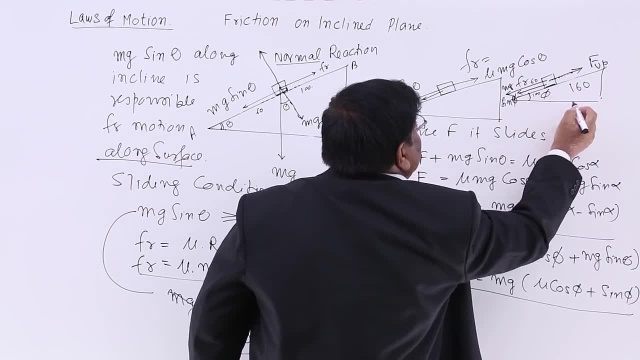 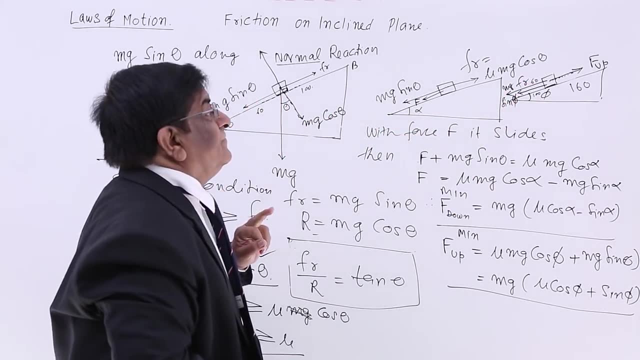 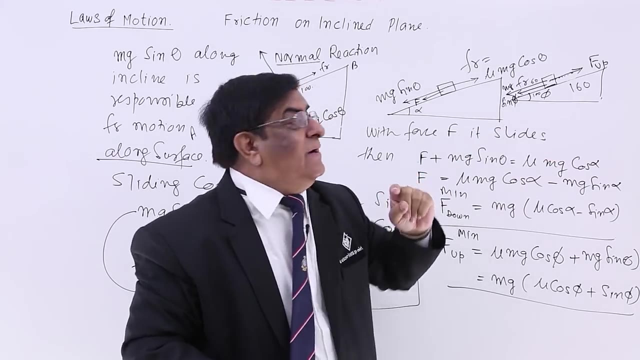 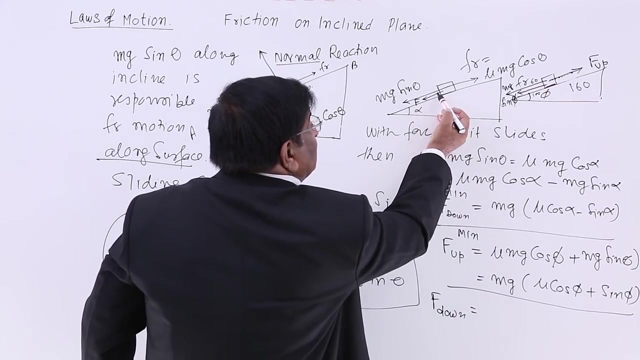 I have to apply. answer: I have to apply 160, 100 to counter the friction 60 to counter mg sin theta. therefore, I have to apply 160, then only it will go up. please remember what did you find the force to bring it down? in this case it was. in this case it was 100 minus. 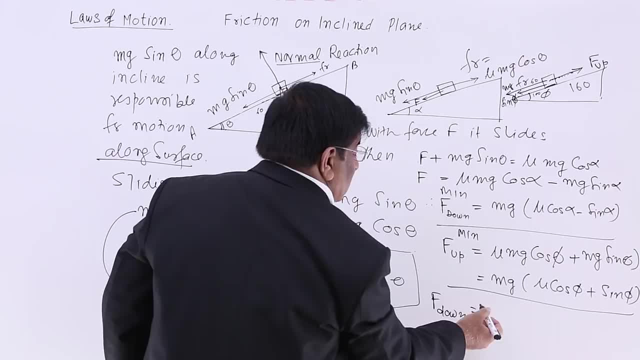 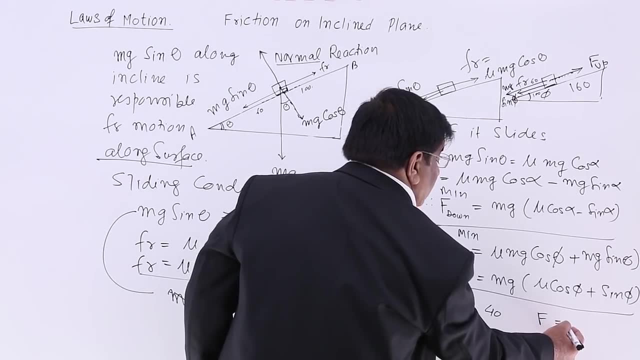 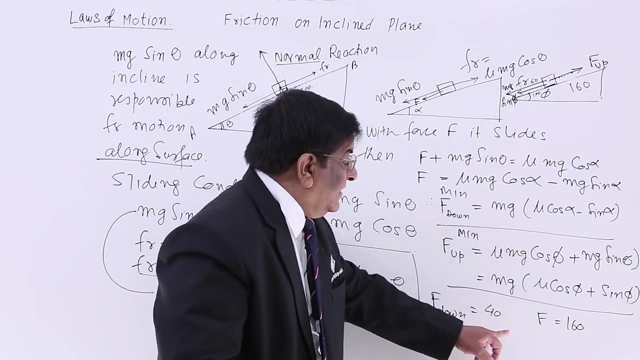 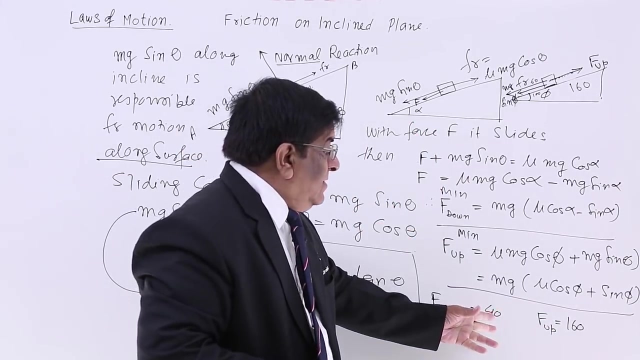 friction minus 60. And that was 40. if I want to push it up, then how much? we have calculated 160. now there is a large gap between the two. suppose I apply a force of 100. then what will happen? 100 upward, it will not move up. 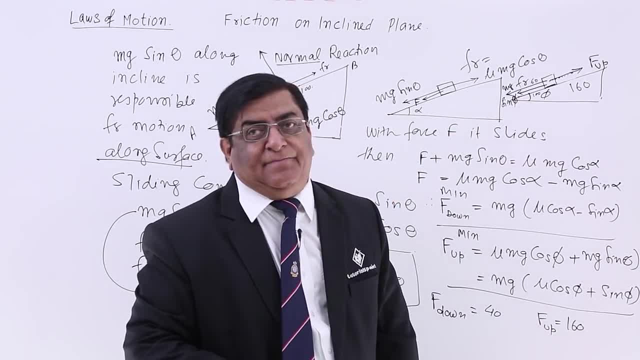 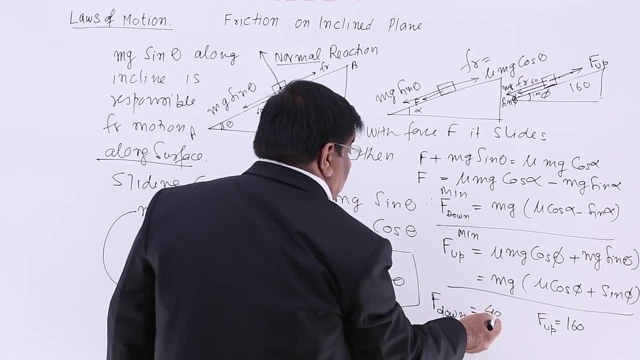 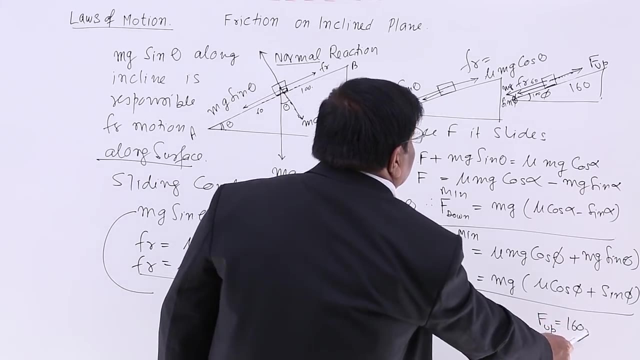 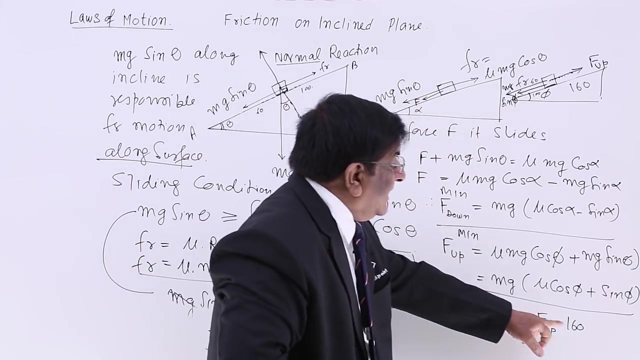 Because up motion start only at 160. okay, I apply a force here. okay, this is 40 in this direction. say minus 40. so minus 40 to 160. what is the situation of this object? minus 40, it will start coming down. plus 160, it starts going up. and what are the forces between these? 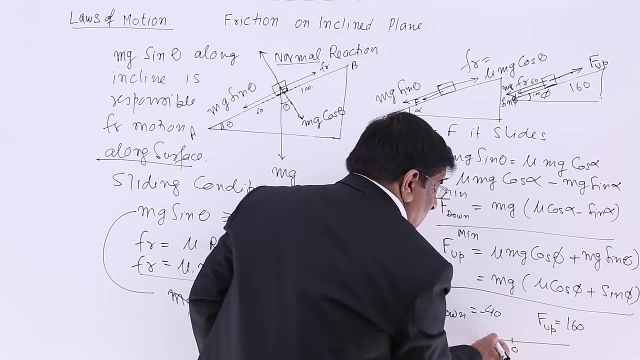 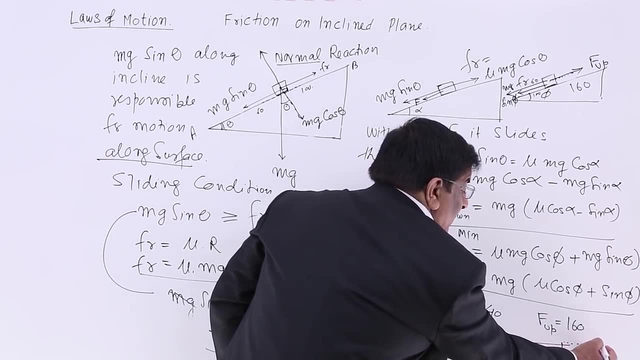 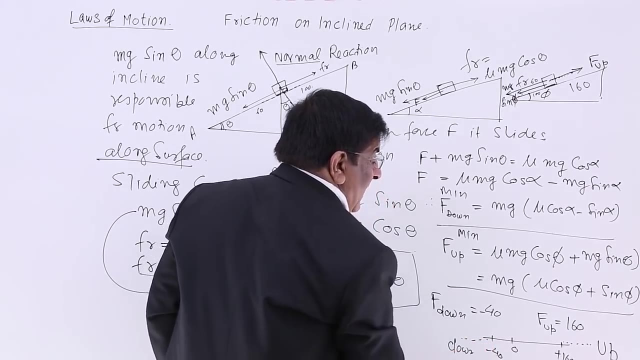 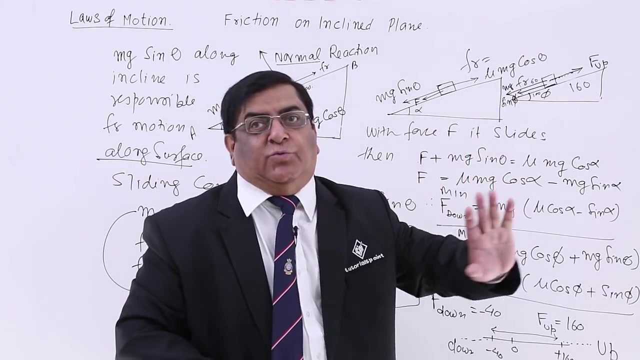 two. This is 0 line. this is minus 40. this is plus 160. if I apply this force, the body is going up. if I apply this force, the body is going down. what happens if I apply force in this range? answer is: the object will not move. so we have solved the question: for what range? 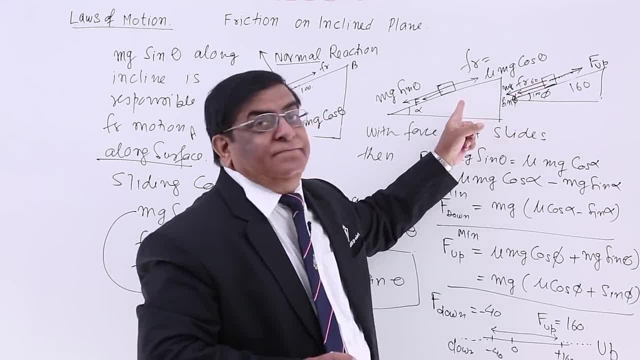 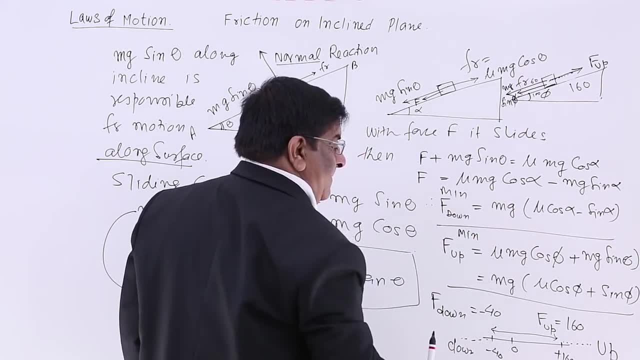 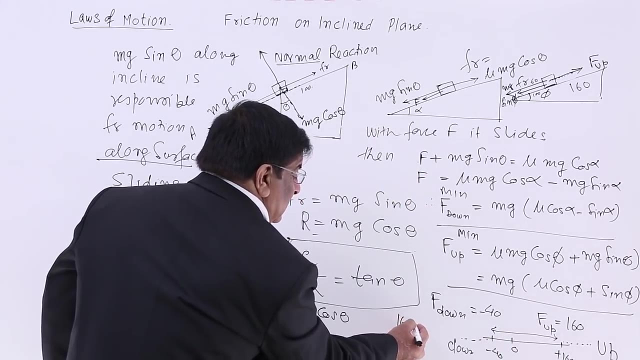 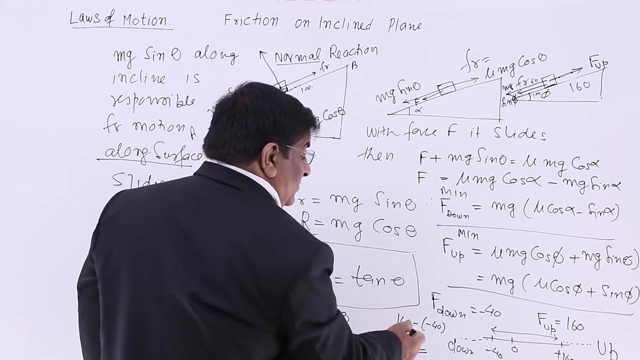 of the force, this body will not move. What is the range of that force? this up minus this, 160 minus minus 40. so this will be 160 minus minus 40. this is equal to 200. is the range? 200 is the range for which this object will. 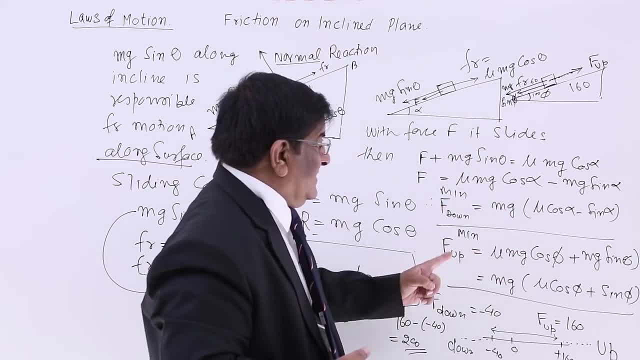 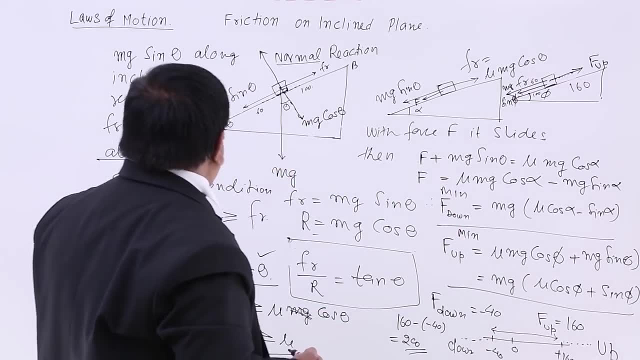 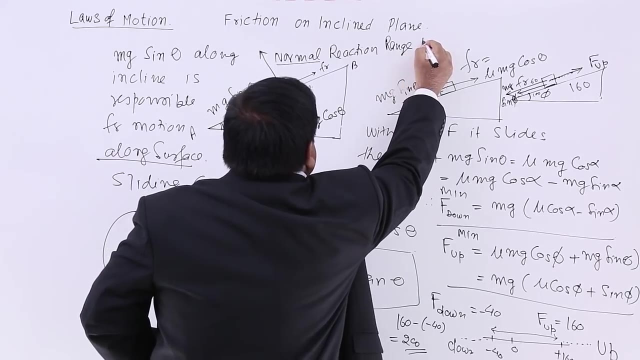 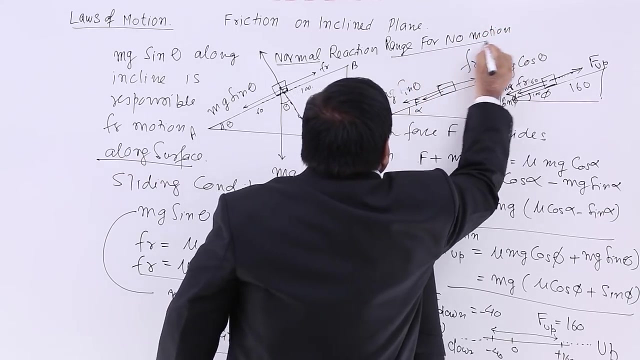 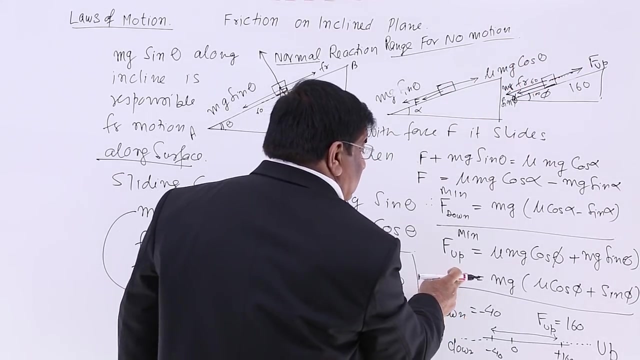 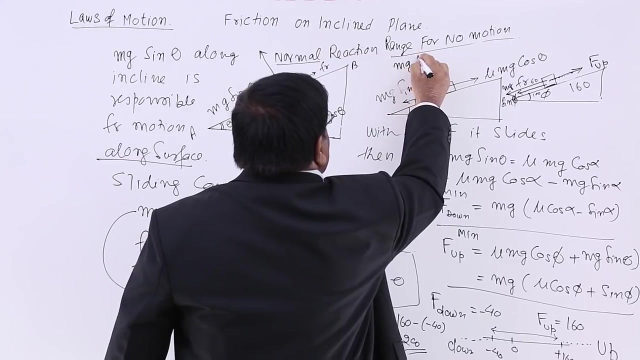 not move. can we make it in these terms? answer yes, this is for up, this is for down. make a minus. so how much it will come? I will have to write it somewhere. range for no motion. the range for no motion. This, let us this minus. this. mg is common, mg is common inside. first I will write this: mu, let 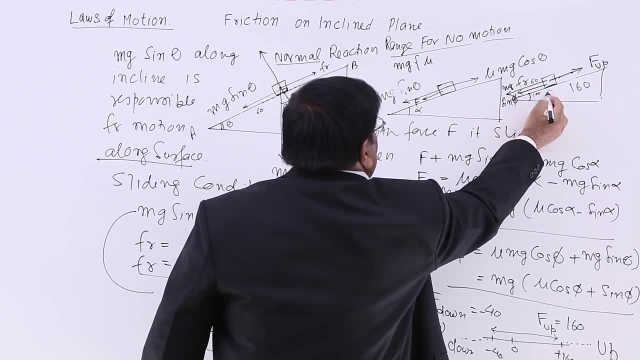 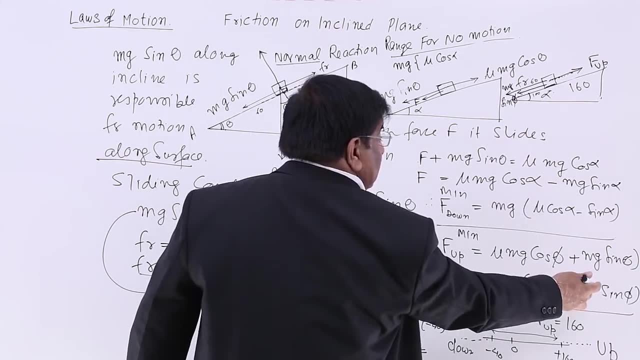 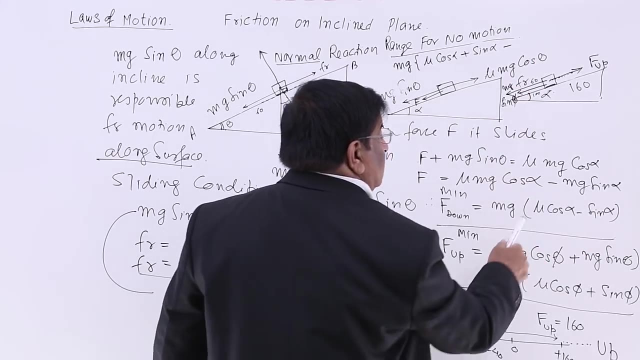 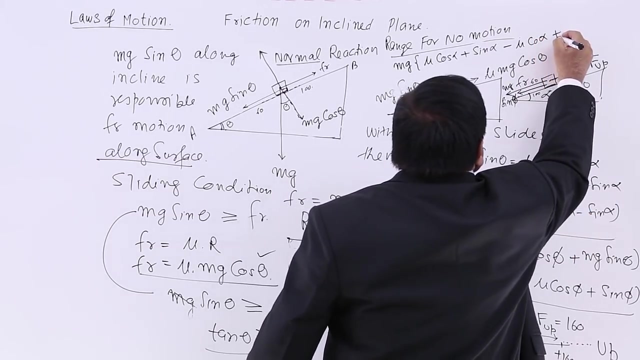 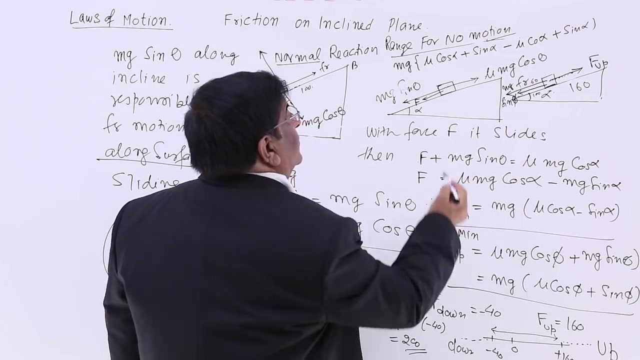 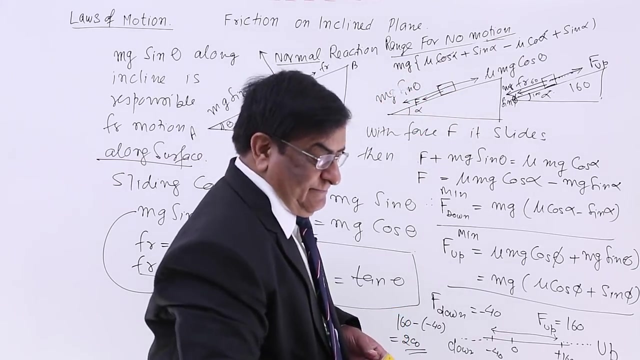 us suppose the angle is same: alpha for this it will be mu cos alpha plus sin alpha. then minus these two terms, this is minus mu cos alpha, and this minus and minus will become plus sin alpha. okay, now you see, mu cos alpha is cancelled. what we get is 2 mg sin alpha.